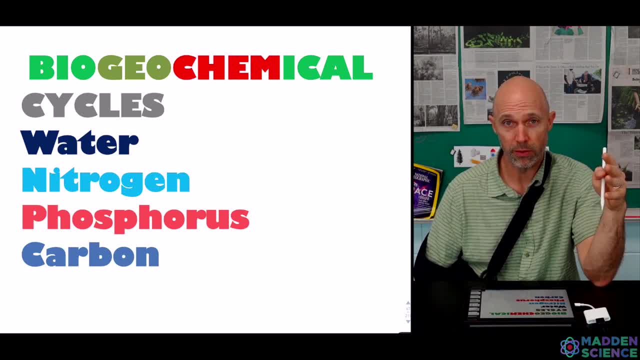 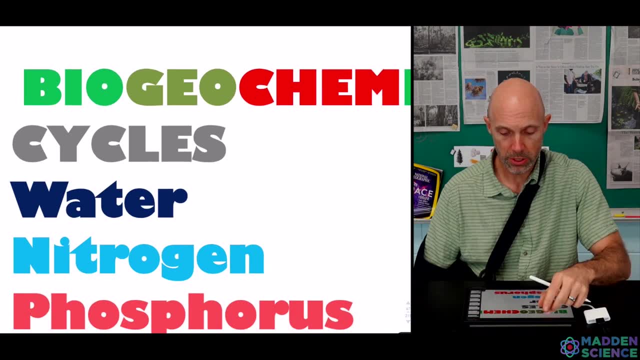 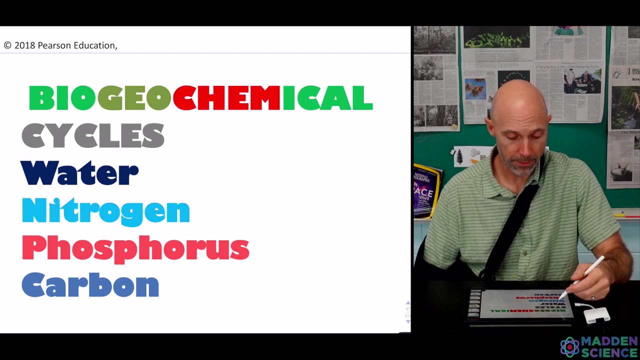 this video and gives us a little bit of an overview of the chemistry involved in the environmental science that we're doing. So focusing on this, we've got biogeochemical, So the life, the earth and the chemistry involved in cycles: water, nitrogen, phosphorus. 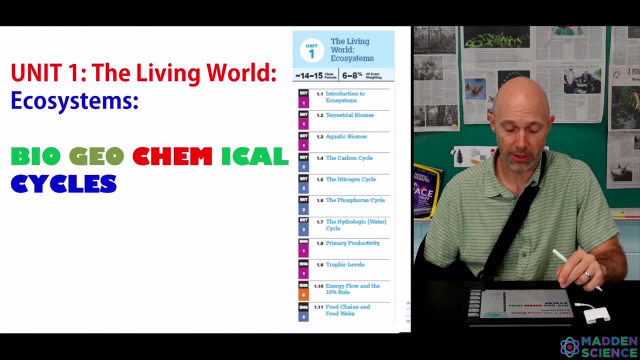 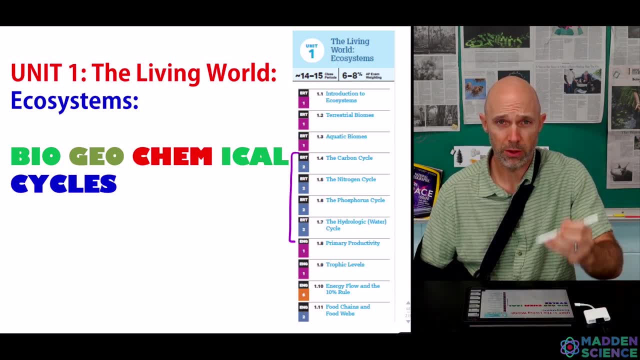 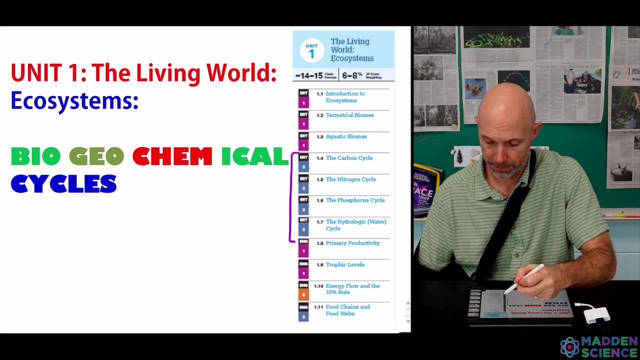 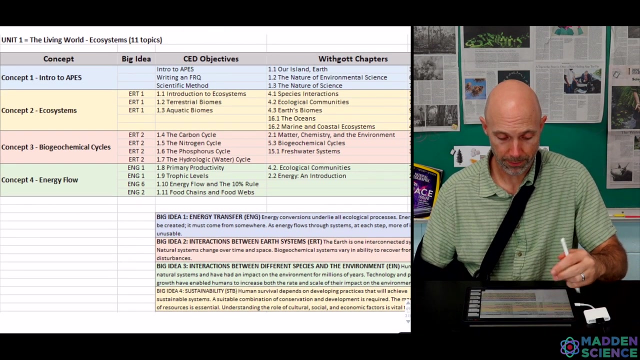 and carbon. Sometimes we call them water, the hydrologic cycle. So we're in this area right here And we'll focus one, followed by another One, two, three, four sections, four through 1.7.. If you look at our CED, we're still in on concept three in unit one. 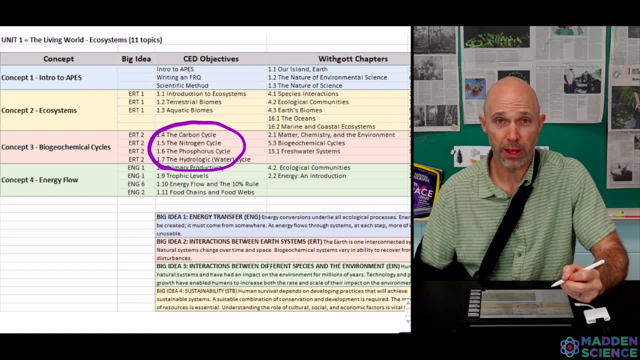 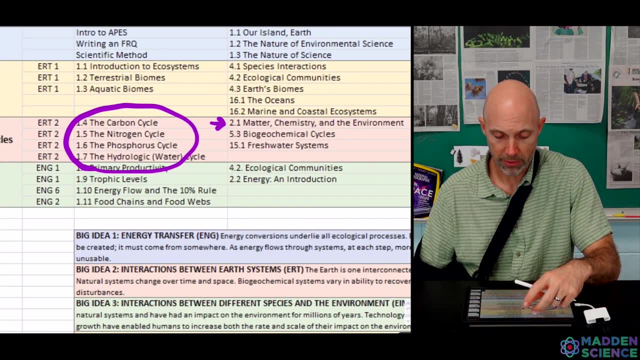 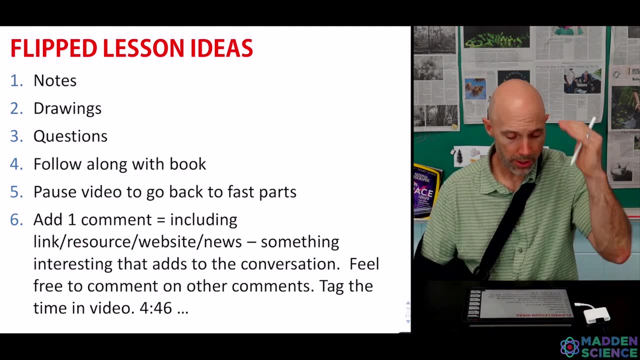 right here. So yesterday's video was focusing on section 2.1.. Where we're at right now is going to be in 5.3. Just a reminder for the flip lesson style of what we're trying to do with this: notes, drawings, writing down your questions probably follow along with. 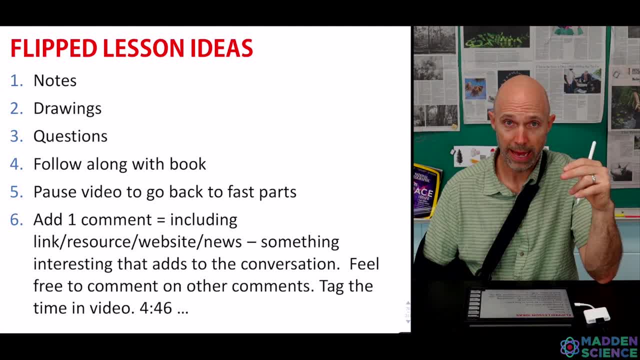 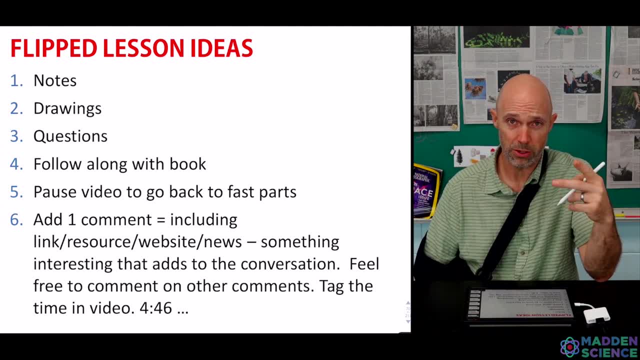 a look. Keep in mind, you can pause at certain points, knowing that, well, I'm going to go through it pretty quickly, Sometimes even just skim past a picture or two. You'll need to take notes and drawings and in the comments, add something. I'll give you a few examples. 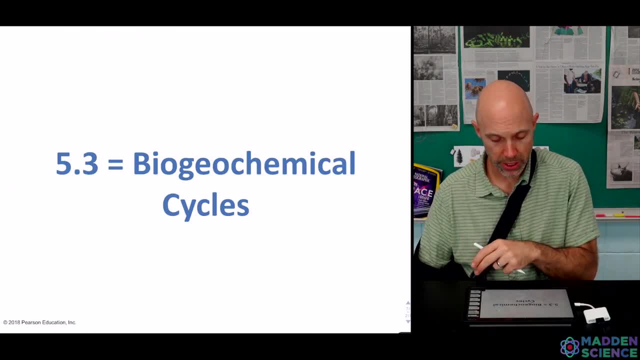 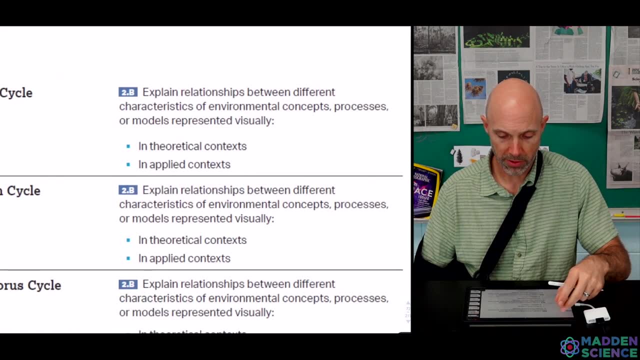 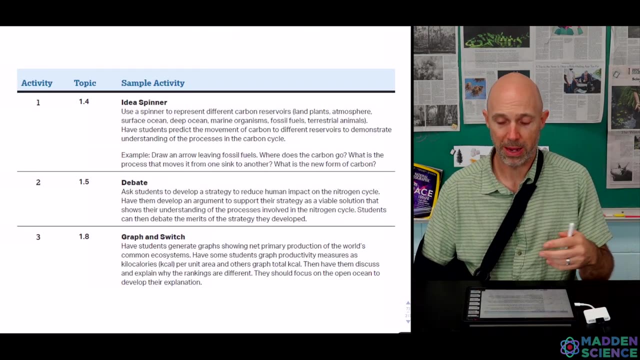 of that as we go. So 5.3, biogeochemical cycles. If we look at the APES, CED, you can see these listed here along with some of our goals and objectives. You can see that those are going throughout. A little more detail on some ideas that we'll do in class You can. 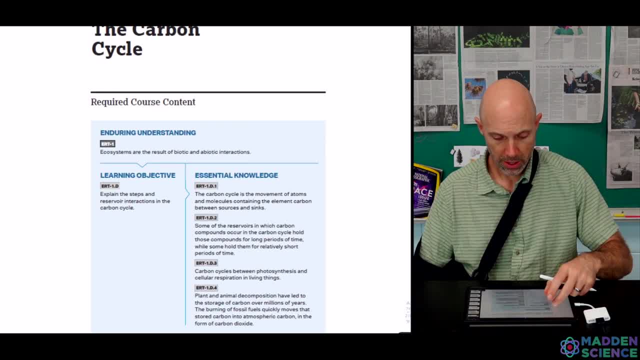 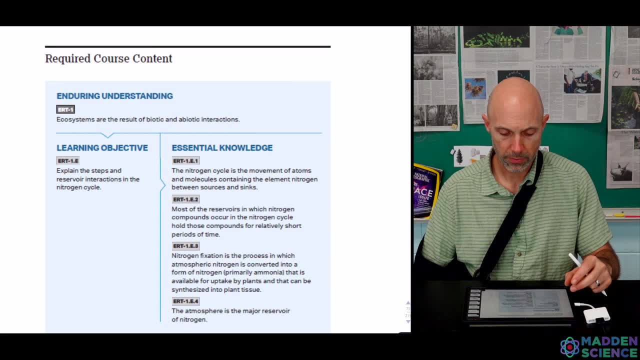 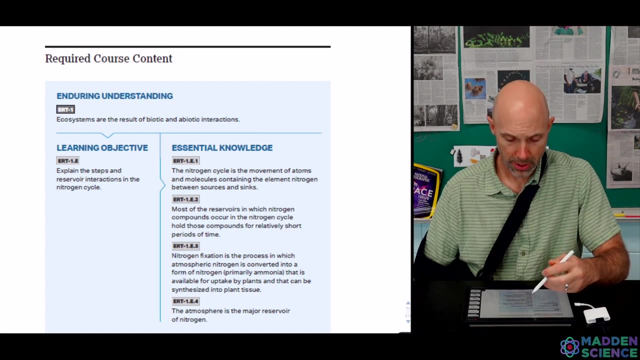 then look at topic 1.4 with carbon objectives and essential knowledge. So that's carbon cycle, nitrogen cycle. Notice that they're pretty similar. So essential element here: nitrogen cycle is the movement of atoms and molecules containing Aliment Nitrogen between 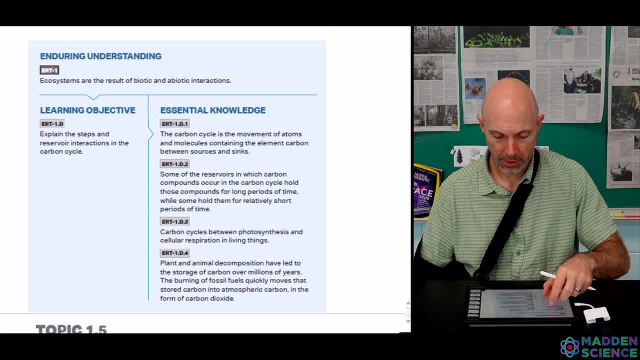 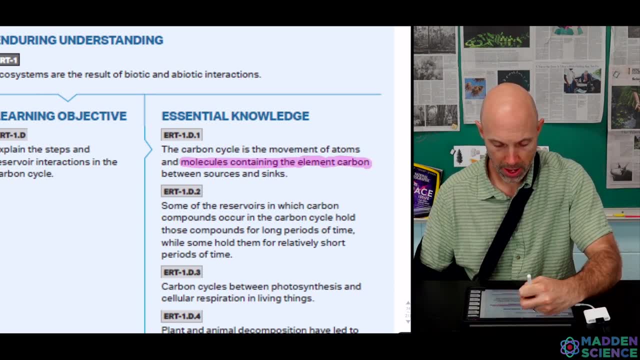 sources and sinks. If you back up, you'll see that- the Liller scale, you'll see this at the center of it. we're going to see the抱mer cycle. languages virtually the same, So molecules containing the element carbon between sources and sinks. So that's going to be an important piece of what we're. 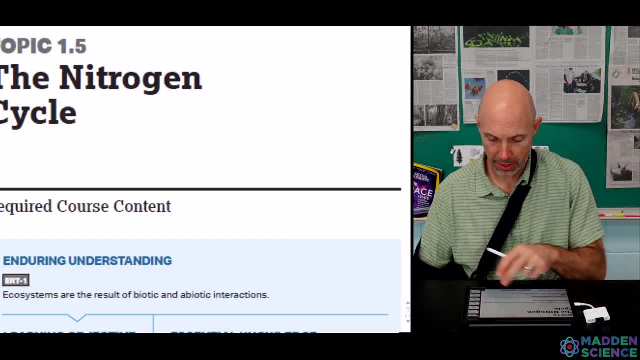 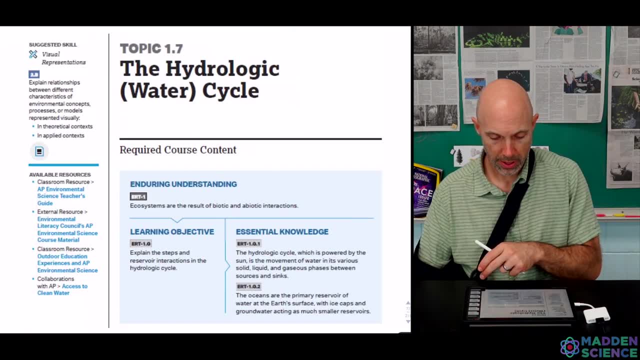 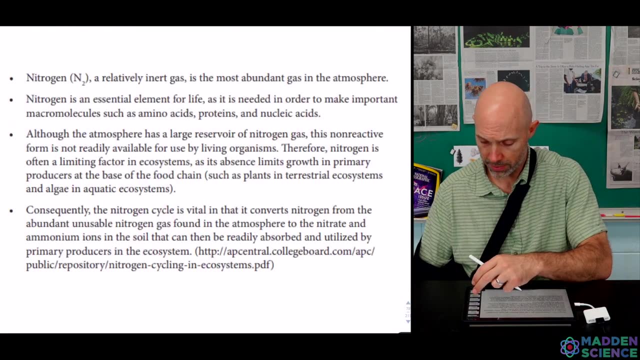 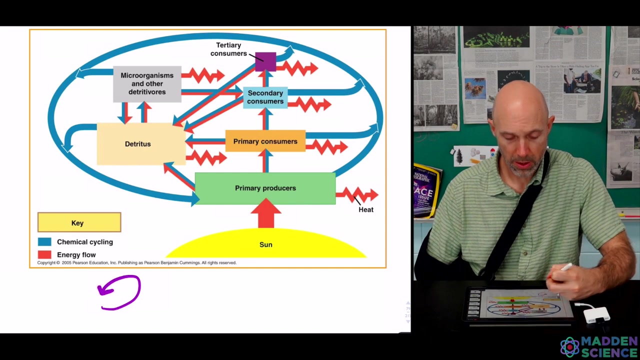 doing is what's a source and what's a sink. So nitrogen cycle, phosphorus and water, or hydrologic. You can see some quick, key facts about nitrogen, reminding us a concept that an ecosystem matter cycles and it's energy that flows. So 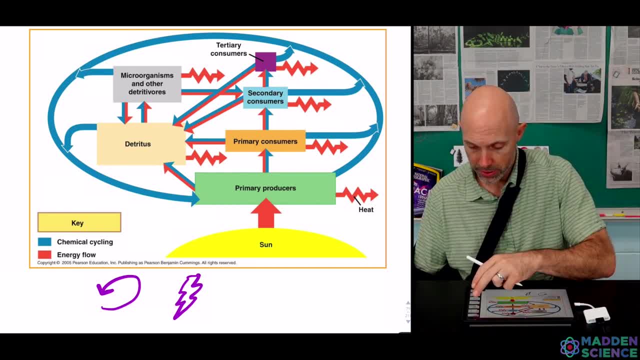 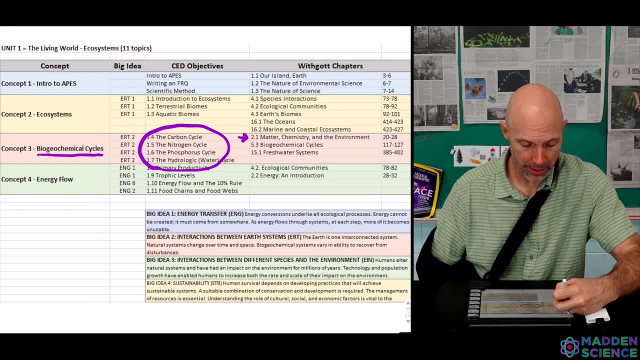 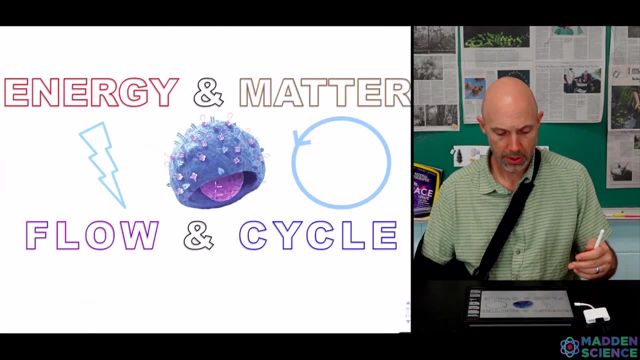 right after this section, kind of if we skip back to here, you'll see that right in here. for biogeochemical, we're in with matter and in concept 4, dealing with energy, Skip back. we got it shown here: can flow versus sink. 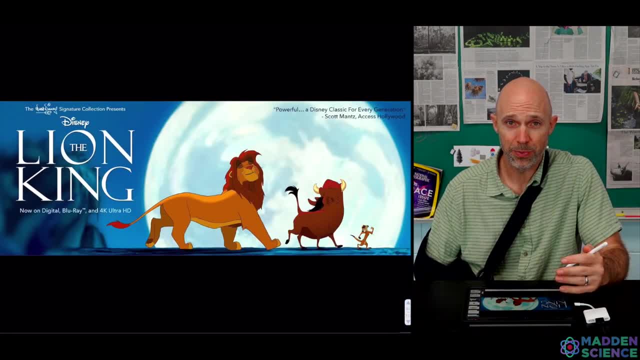 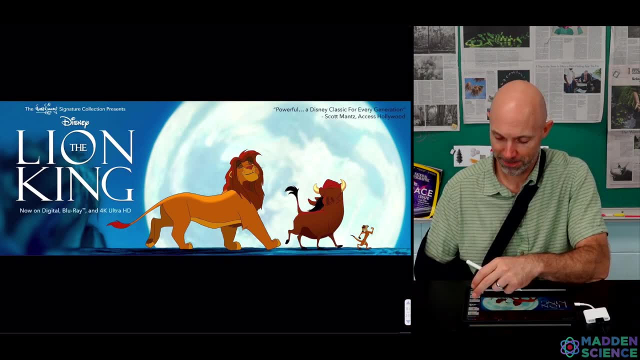 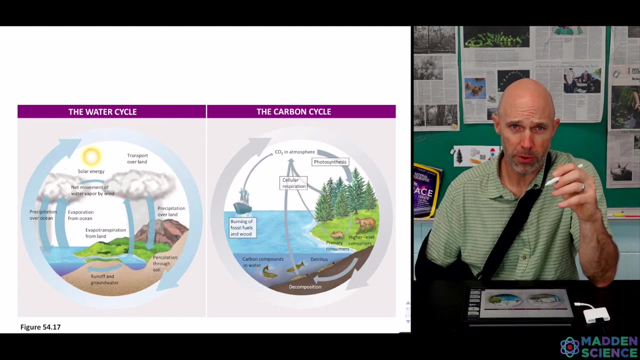 cycle. Can I say Lion King, Hakuna Matata, cycle of life or circle of life? I should probably edit that out. Here's one quick view of our different biogeochemical cycles. We'll go basically in this order. It's also important to note that your 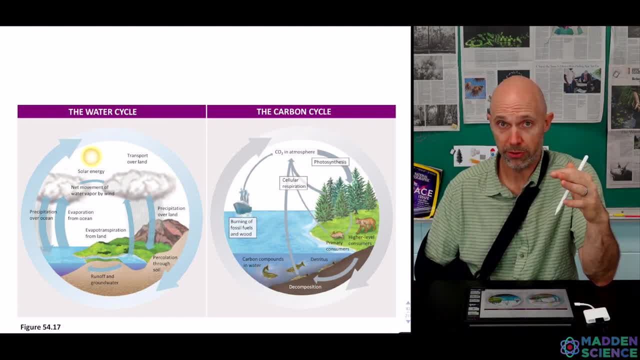 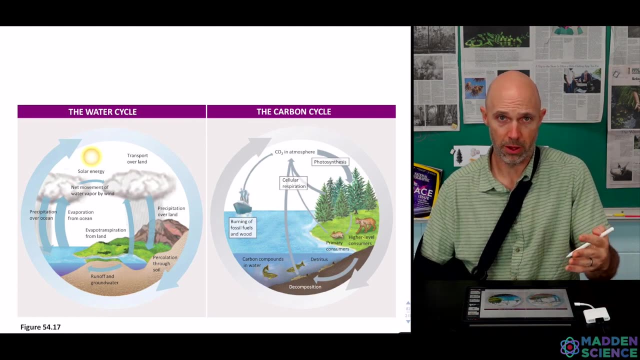 book has some really cool biogeochemical or nutrient cycles, because it shows the amount. So it gives that amount in, say, kilometers, cubed or teragrams or petagrams. Not every book has that, So here's some other pictures. Also, your biozone has another alternative view, So certain views leave one thing out or 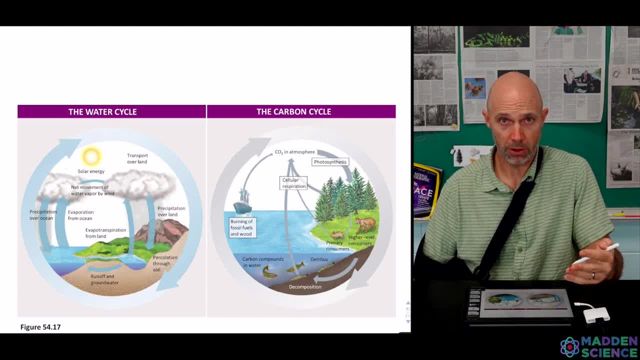 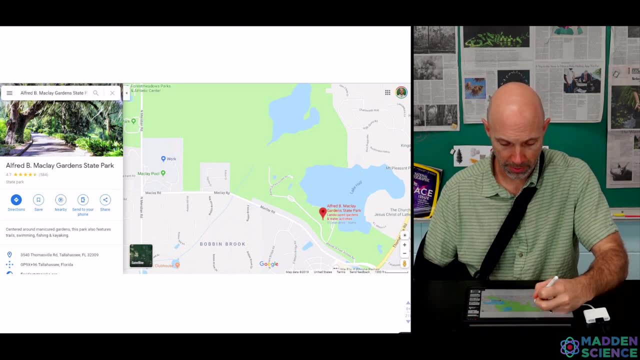 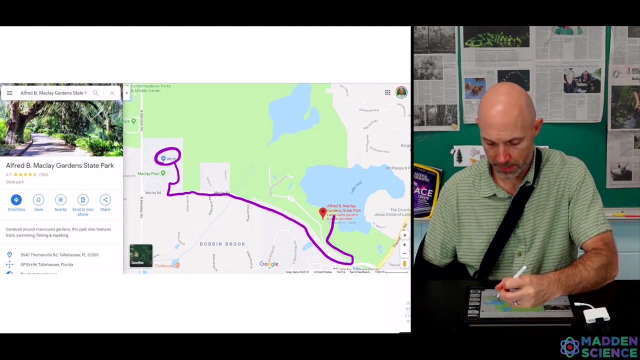 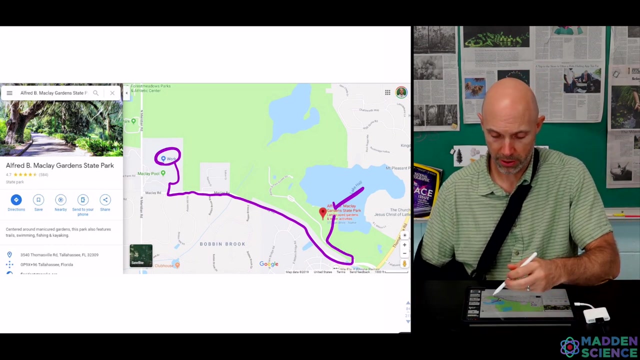 another. They highlight certain sources or sinks or maybe the flux. One thing we'll be doing soon will be traveling, So from school, and we're gonna go check out and try and experience nutrient cycles, doing some testing of water and soil and biodiversity over at 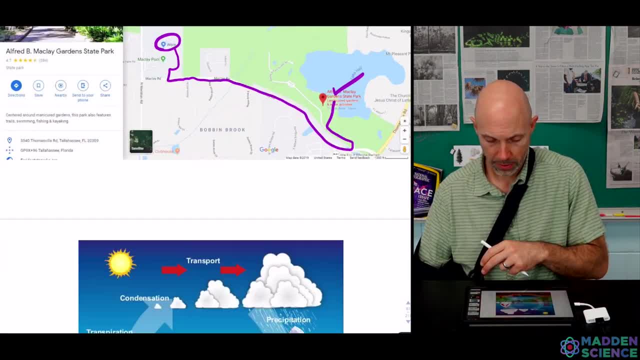 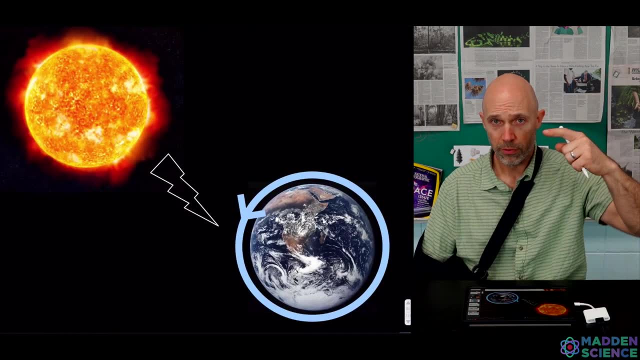 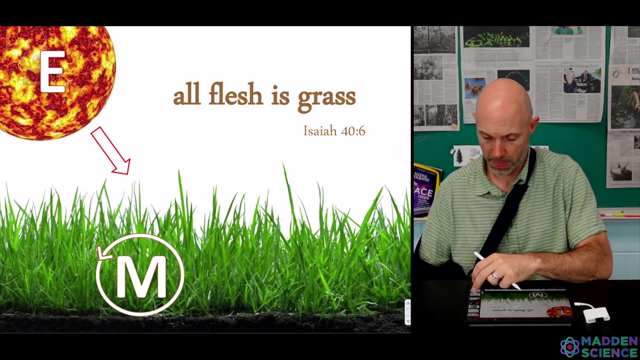 Lake Hall at McLean Garden State Park. Here's a cool picture of water cycle, Again an image for flow versus cycling nature. We're reminded that all flesh is grass. So we build up and up, In particular with carbon cycle, the connection between photosynthesis and cell. 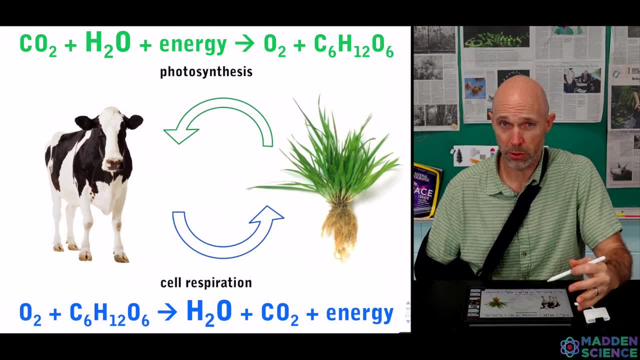 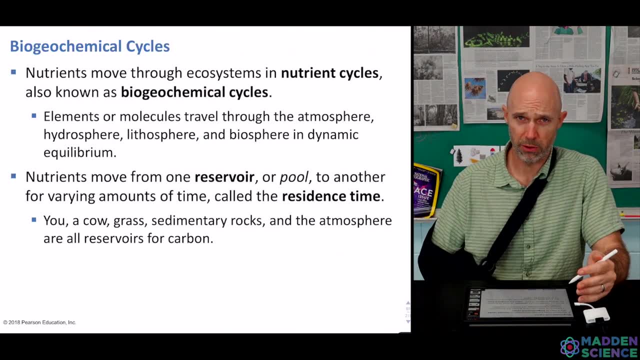 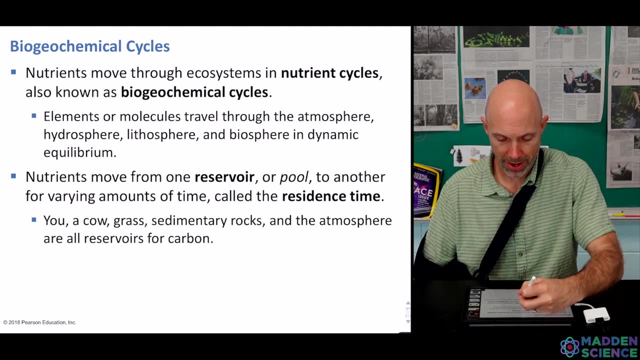 respiration, Like we did in class. you're gonna want to be able to build these equations. Make sure you understand the formulas, how they work. These are in the unbalanced form. So in general for biochemical or biogeochemical cycles and nutrient cycles, we got important terms here with the reservoir or pool. 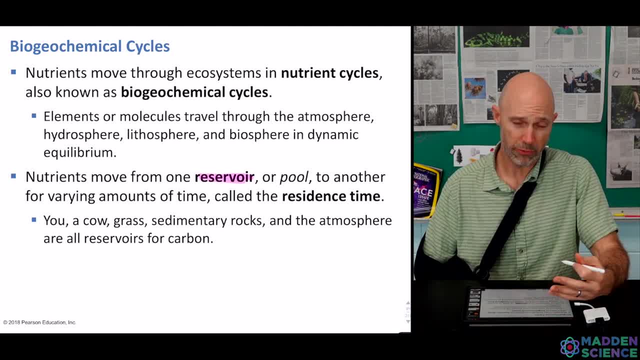 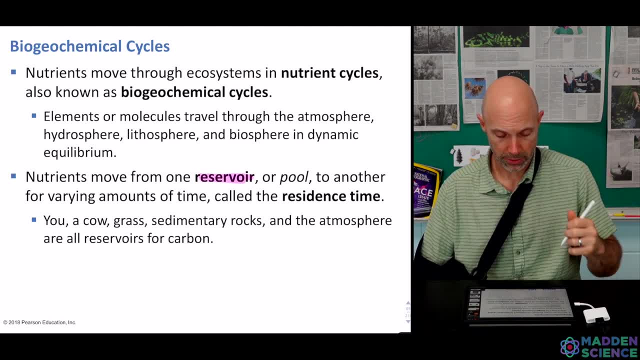 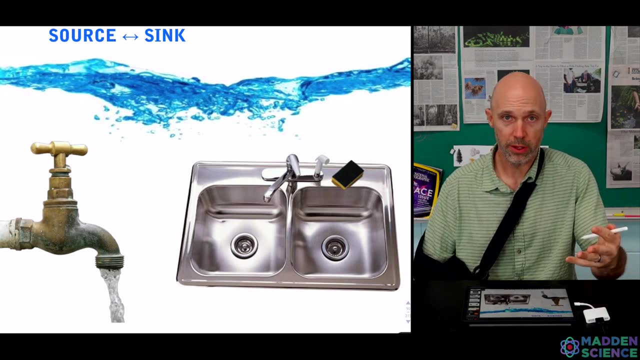 where those elements, those nutrients are stored. And for our case, with the four, we've got carbon, nitrogen, phosphorus as elements and then water as a molecule Source and sink. So where there's movement out or loss of be a source and a sink where there's storage. You probably hear these terms most often with carbon. 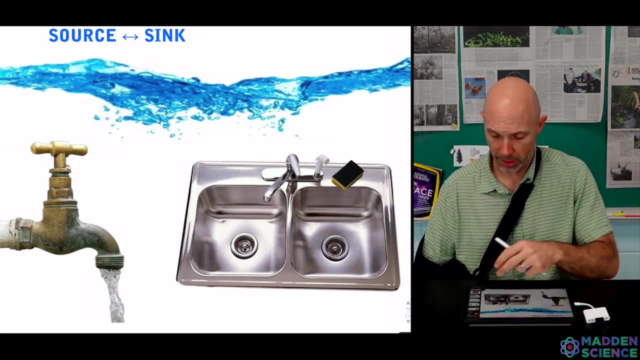 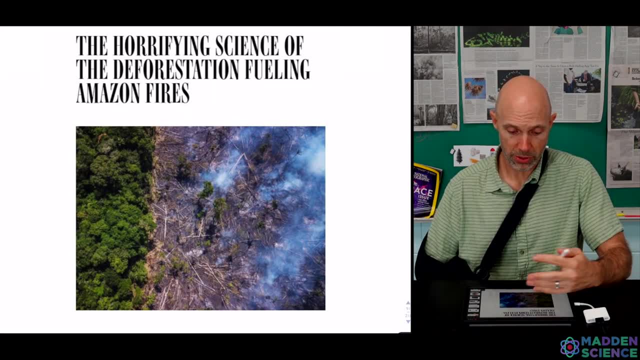 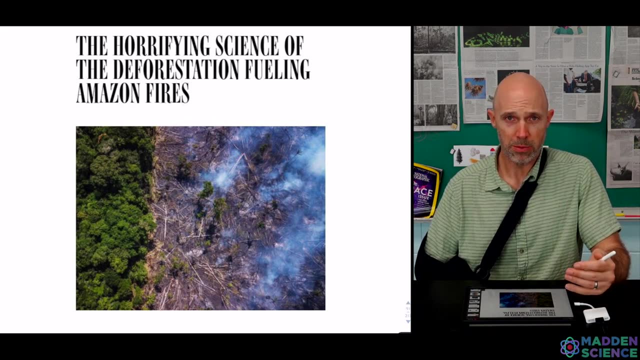 cycle and in relation to climate change, which we've already talked about a bunch this year, Particularly with Amazon fires and the way in which the edge effect is creeping in and degrading, causing a disturbance and making it harder for Amazon to sequester carbon or to serve as a sink. So you're actually getting 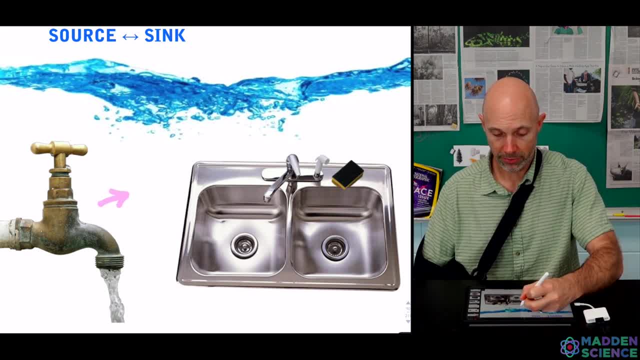 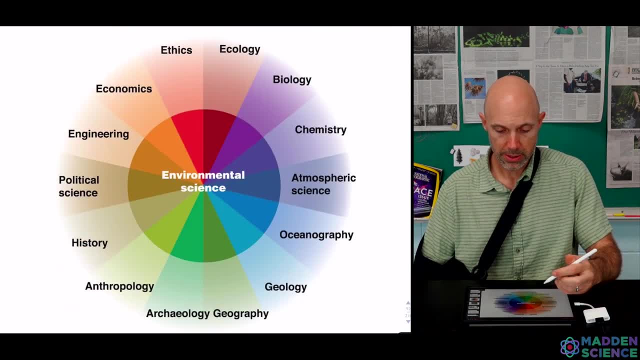 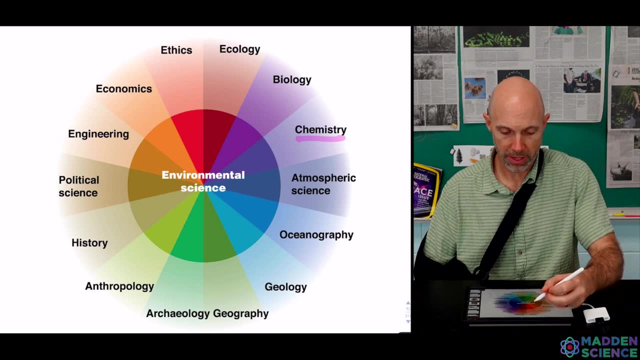 more outflow of carbon and less storage. So these issues clearly tie into environmental science as a whole, Tie into ecology, biology- Right now a big focus on chemistry and atmospheric science. Certainly a little bit of ethics that will come into play. Political science. This is an image showing you. 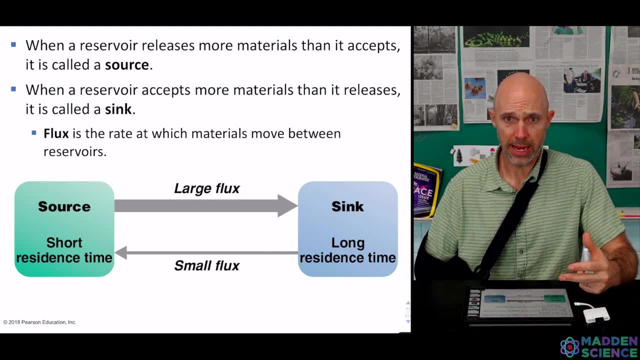 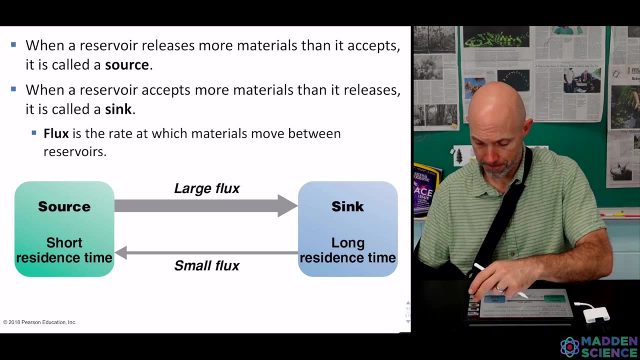 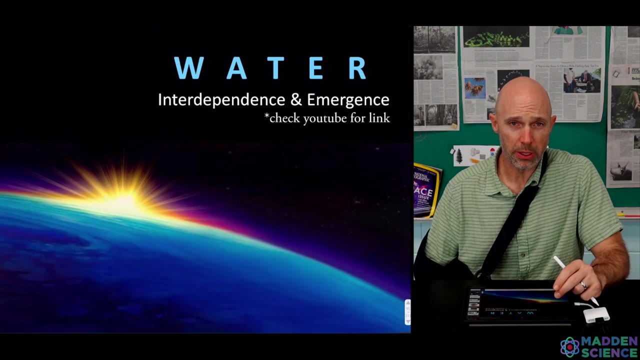 know how long an element or a nutrient is staying in a source or a sink. Obviously, you can have differences in the flux or the transition from one to the other. Again, this is changing pretty regularly, perhaps yearly, seasonally, daily. We'll start first with water, So the hydrologic cycle or the water cycle. 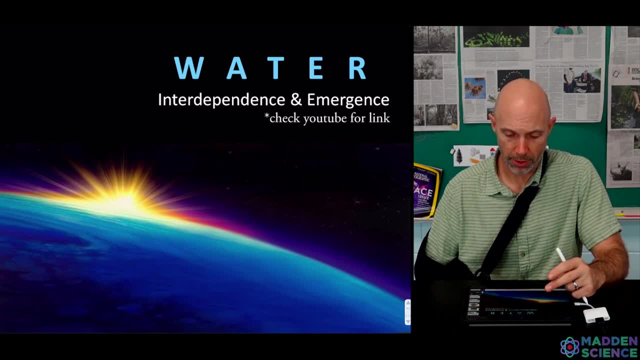 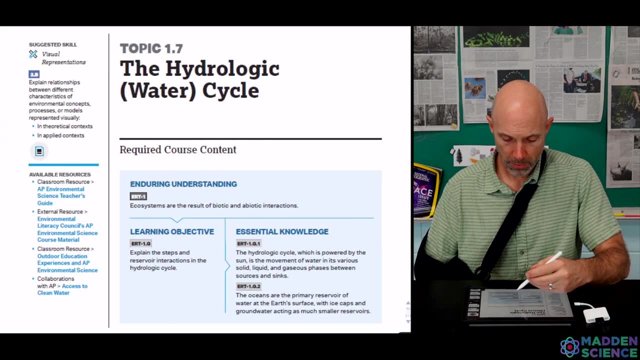 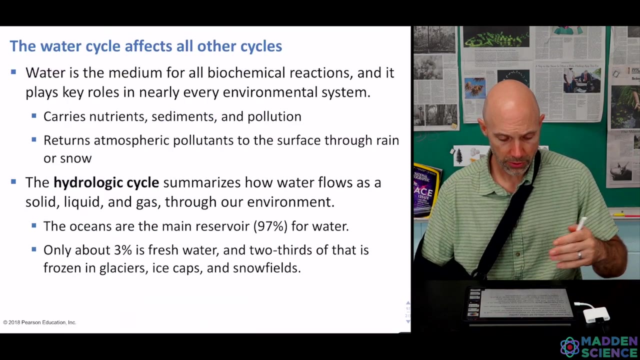 I'll put the link down here. A few years ago I gave a talk and my old school on water Interdependence and emergence- you can check that out below. here again is from our apes, ced breaking down our objectives. you can see for learning objectives and essential knowledge shows most of the things that you already know. 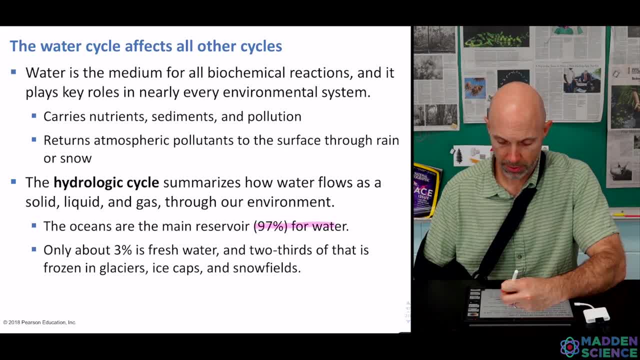 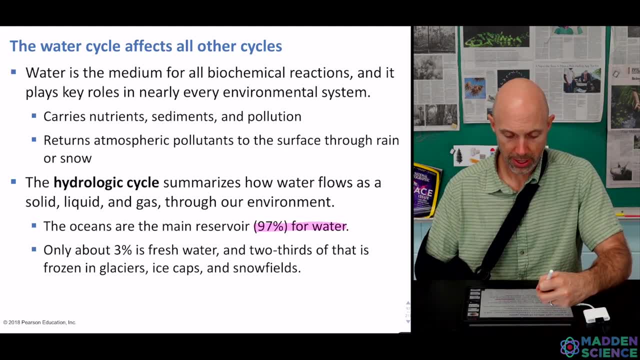 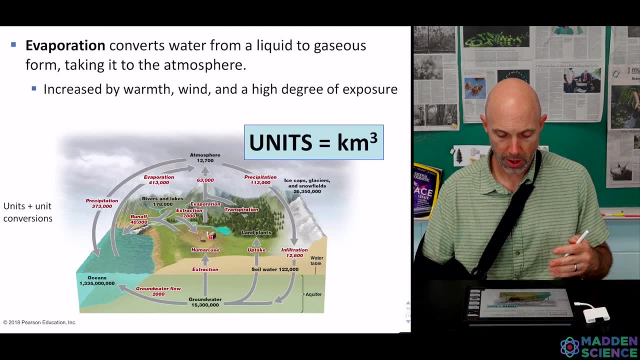 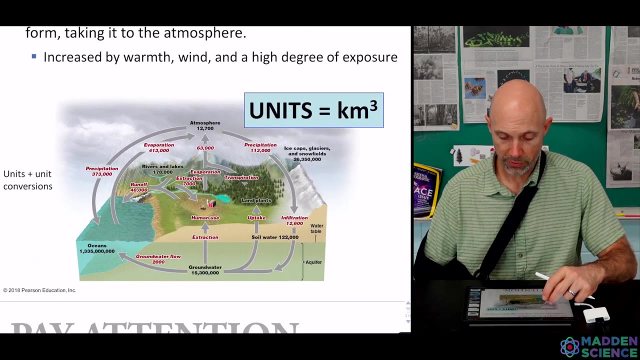 some key stats. ocean is the main reservoir, holding probably 97.5 percent of all water on earth. again, three or so percent is fresh and two-thirds of that is locked away. glaciers, ice caps, snow fields- here's a good view of the cycle in our book. notice that you have reservoirs in black. 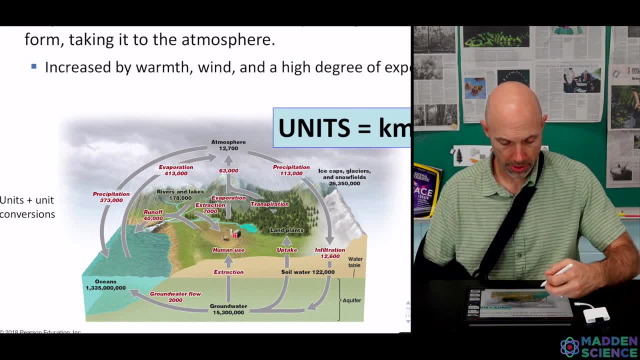 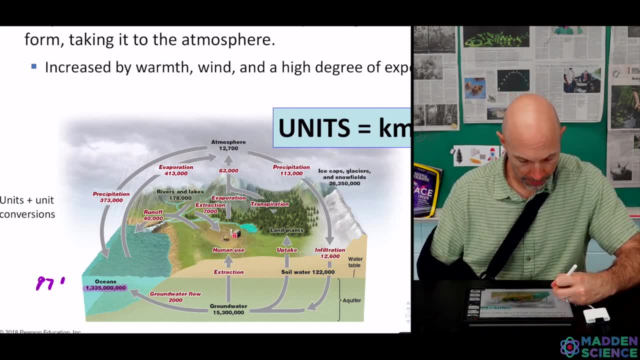 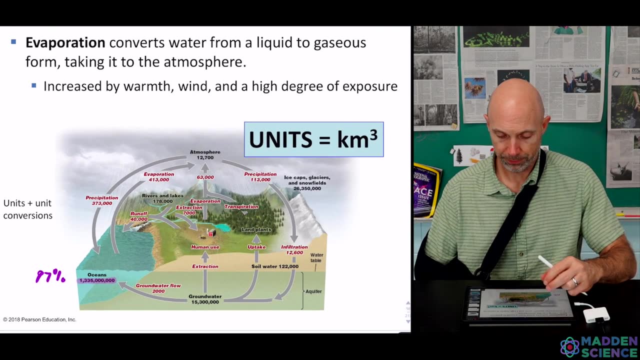 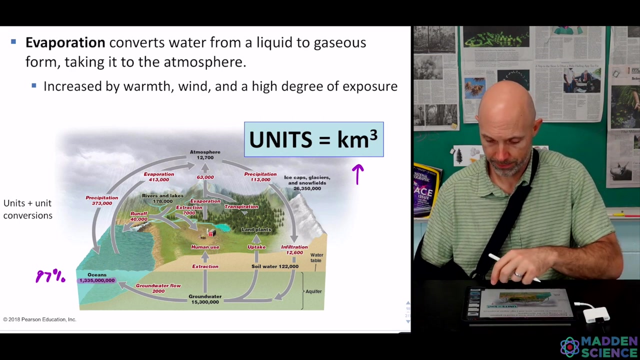 and you have flux in red. note the amounts here. just an insane amount: 97 percent in the oceans and everything else can be around three or even less than three. the units in here are in kilometers cubed, which is pretty hard to fathom. we'll do more on that in a minute when we do some apes math. so again, when we do these, we 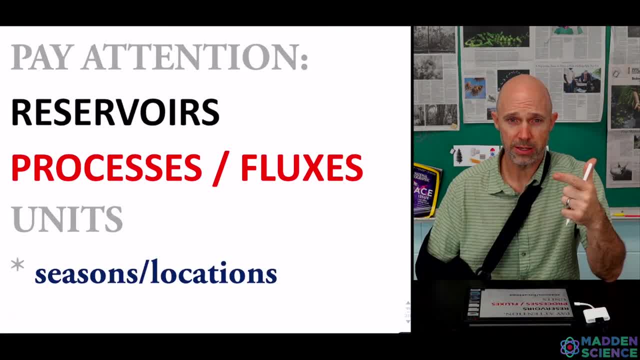 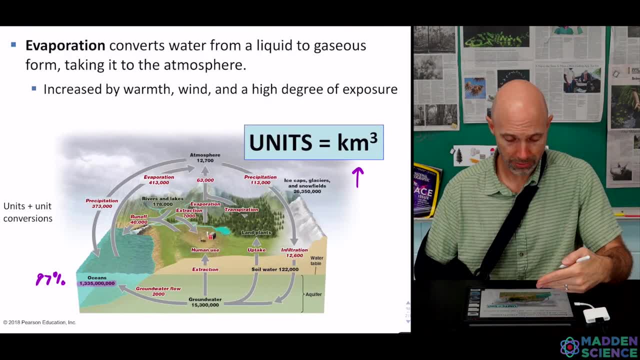 want to pay attention: reservoirs in black, processes and fluxes in red. what are our units? and also keep in mind that even as you see these, that's one place. clearly, not everyone or every place looks like this. this is a tallahassee, for instance, so we want to keep. 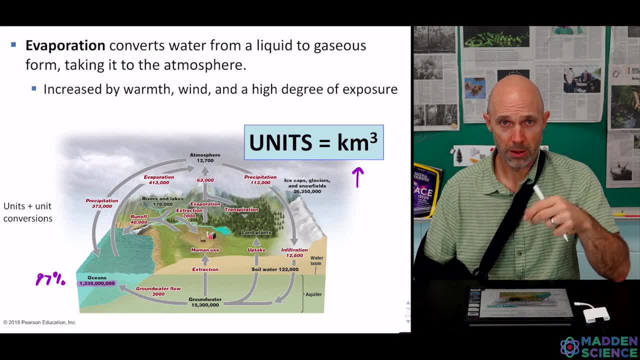 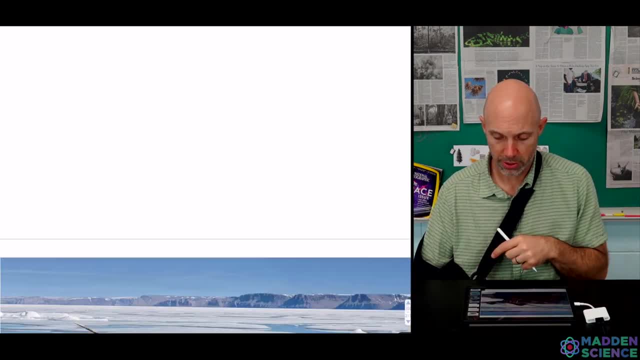 in mind that there's a lot of water in the ocean. so we want to keep in mind that there's a lot of water in this area, so it's important to make sure that we do some changes possible for these guys based on season and location. our units very important here. i want to just show you some pictures. these are from: 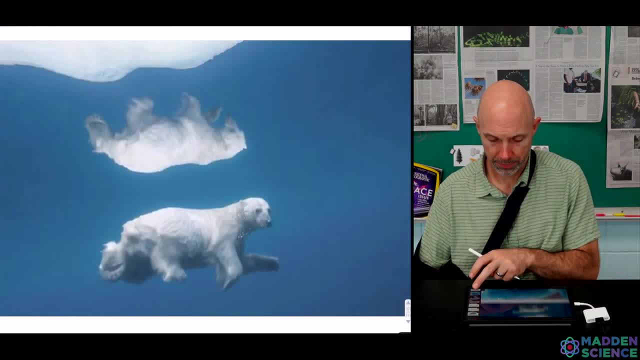 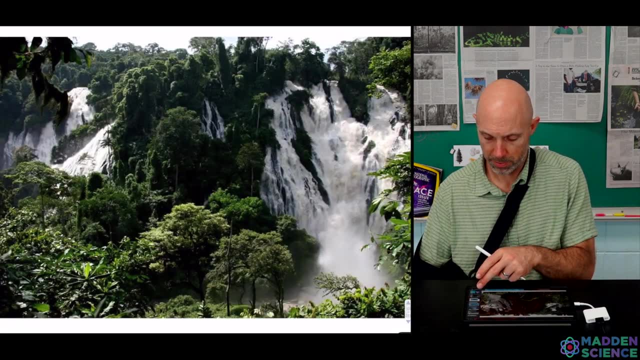 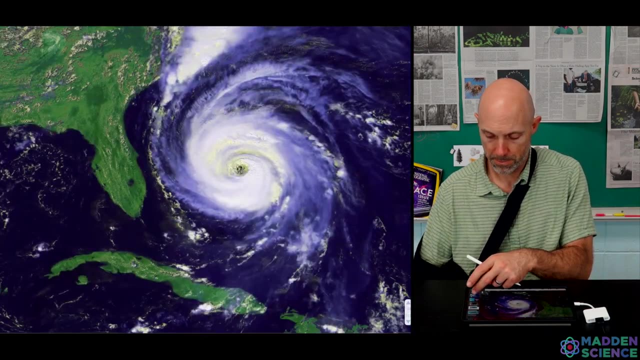 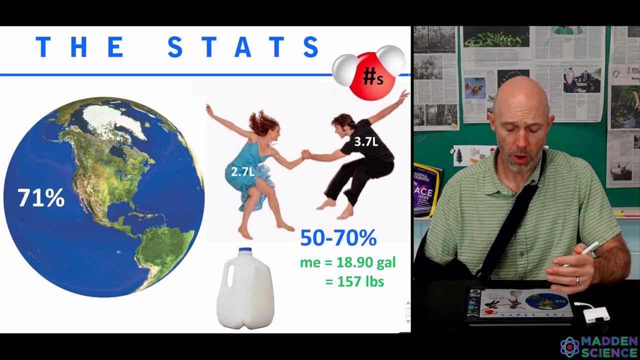 paul nichlin, wildlife photographer, works for national geographic. pretty awesome: narwhals, polar bear, a kitty wake. i think that's a harbor seal. these are separate pictures again showing the importance environment for their stats. we got the planet about 70% or 71% water typical. 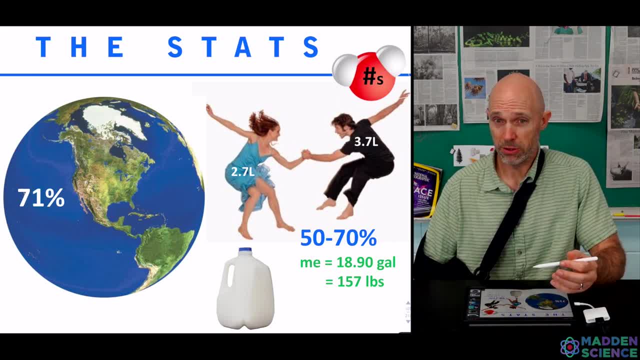 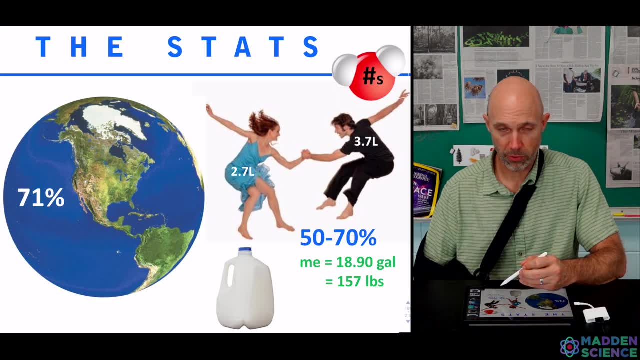 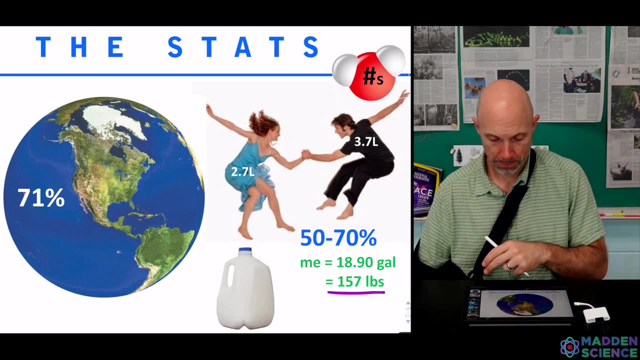 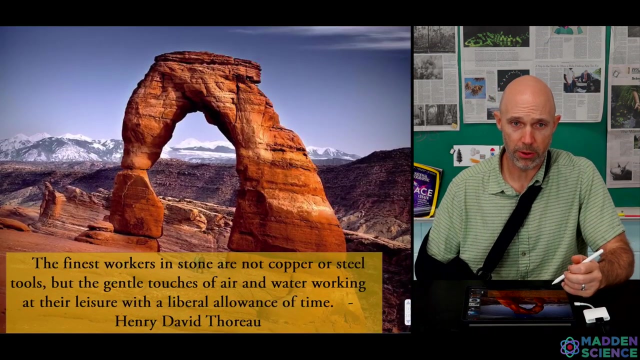 male might have around 3.7 liters 50 to 70% water. for me I've got 18.9 gallons of water and 157 pounds of water just in me. some interesting quotes from old and sacred texts and from authors, and Henry David Thoreau, who said: finest workers in 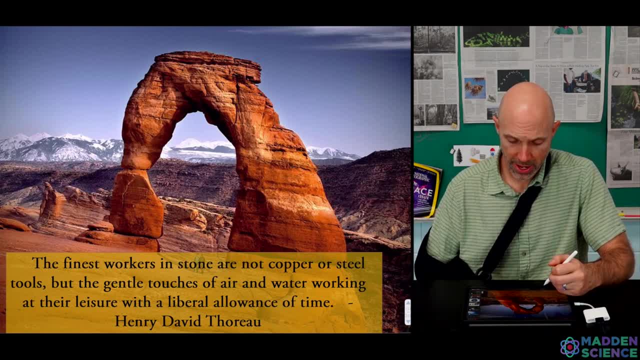 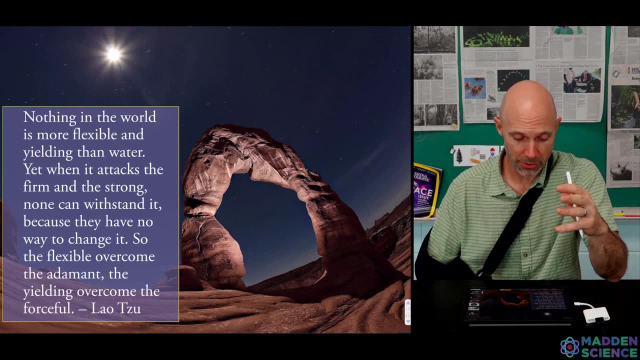 stone are not copper, steel tools, but the gentle touches of air and water, working at their leisure, with a liberal allowance of time, or maybe even cooler, with Lao Tzu who said: nothing in the world is more flexible and yielding than water. yet when it attacks the firm and the strong, no one can withstand it, because 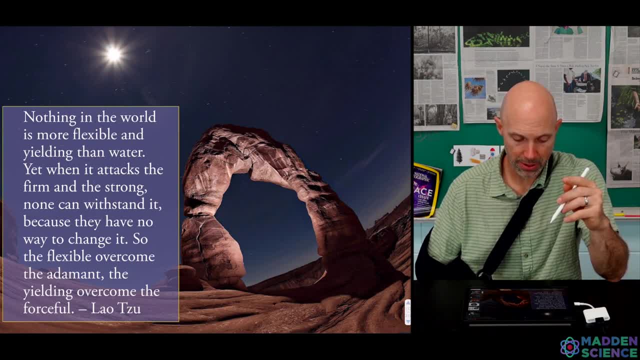 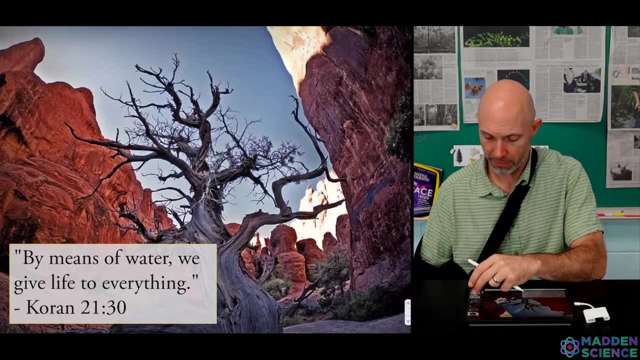 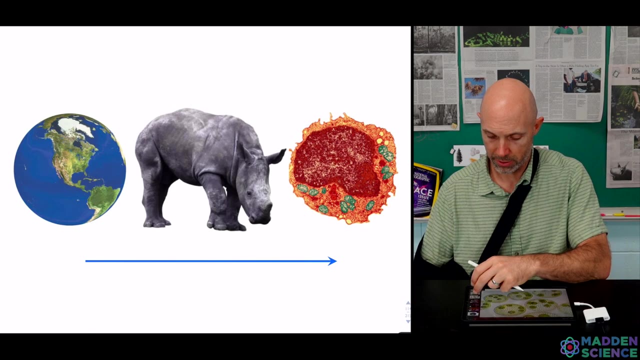 they have no way to change it. so the flexible overcome the adamant, the yielding overcome the forceful, or even here, by means of water we give life to everything. the importance of water goes not just for the biosphere, but to animals all the way down to ourselves. so a few more beautiful pictures showing 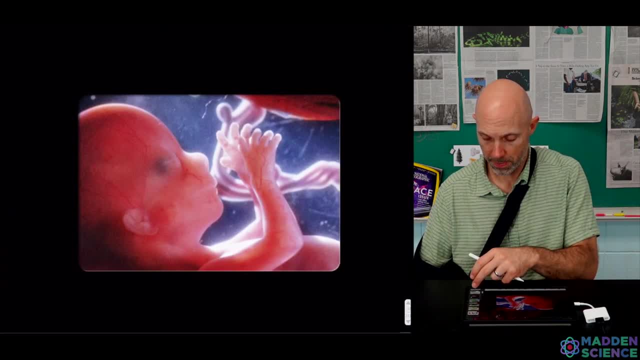 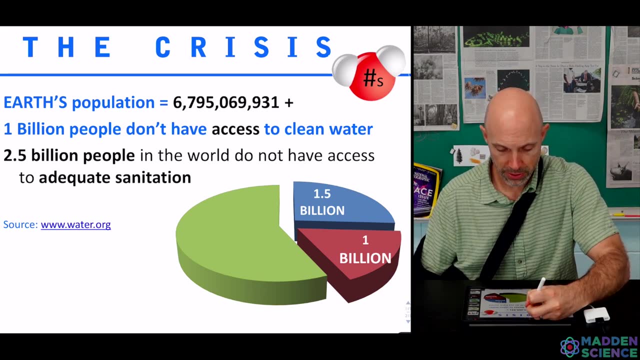 the beautiful and wonderful diversity of life you. it's also a major crisis ongoing with water around the world- probably need to update that population. so we're now around 7.3 billion- more than Billy- don't have access to clean water. you can see some of the breakdown there from water. 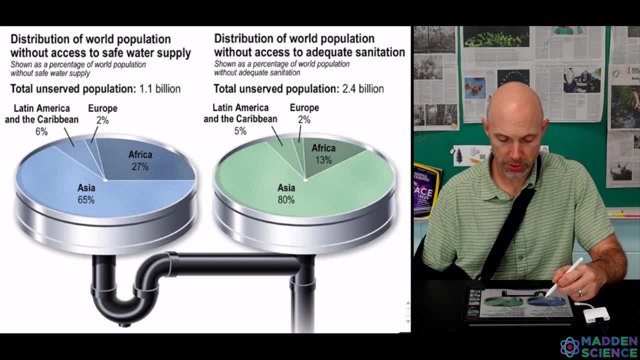 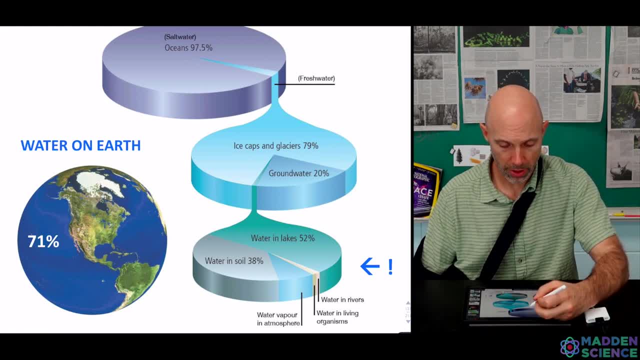 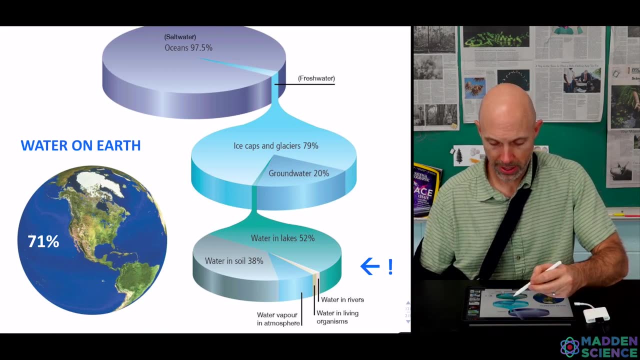 org. further breakdown shows that distribution by continents. you can see, as we mentioned before that reservoir, the ocean coming in and out of the water, the ocean coming in and out of the water at over ninety seven percent, and then the breakdown even further: nearly all of that in ice caps, glaciers and groundwater and then just a tiny sliver. 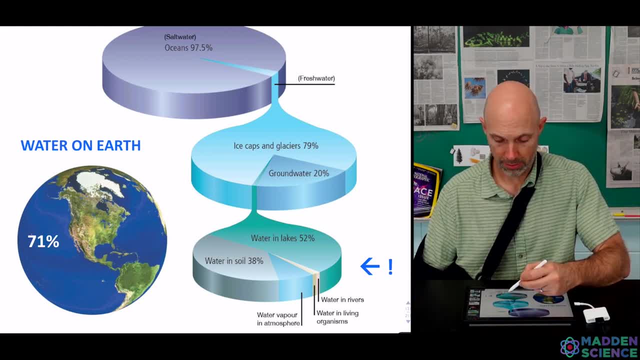 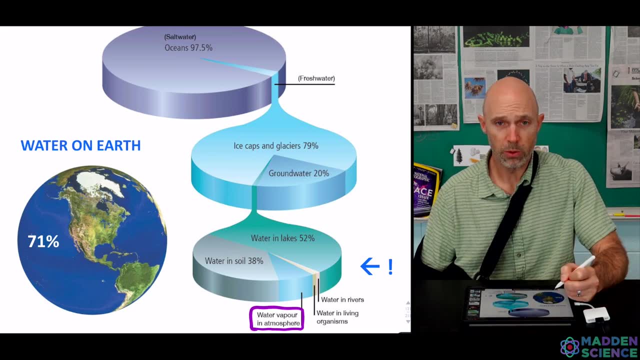 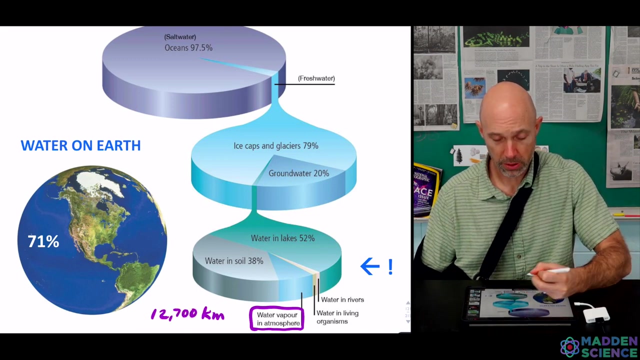 of that to me in lakes, soil and more accessible. keep in mind just this water vapor in the atmosphere, which is even in itself a tiny percentage of the total water, but also an amazing amount of tickets. It's 12,700 kilometers cubed. We'll come back and see what that means. 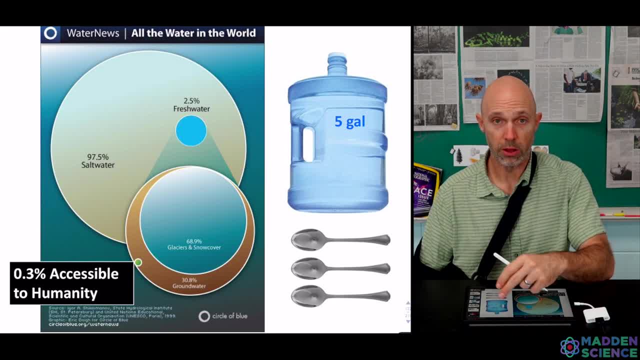 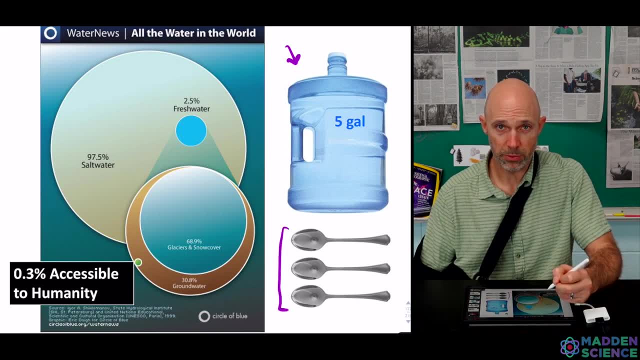 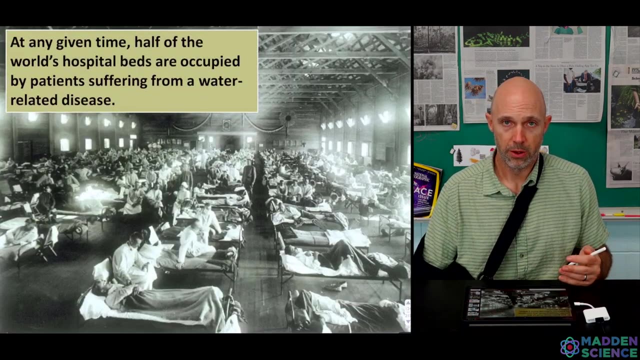 Again, just another way of viewing that. So if all of the Earth's water were in a five-gallon jug, you'd have only three tablespoons of fresh water. So water delivers life, but it also can deliver death, And, horrifyingly enough, at any given time. 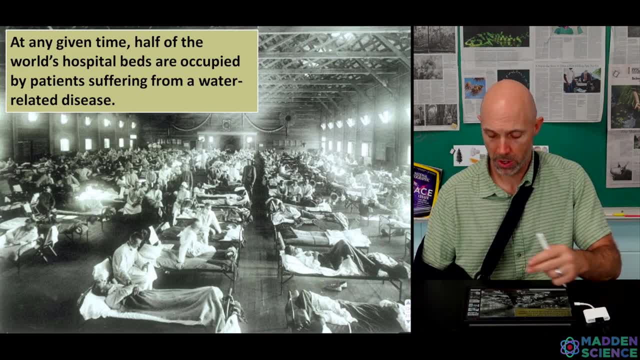 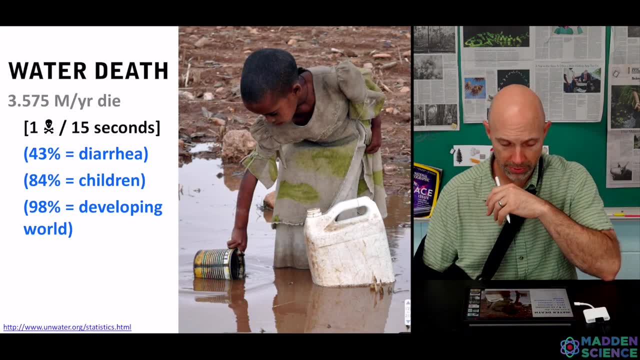 maybe half of the world's hospital beds are occupied with patients suffering from water-borne and water-related diseases. It accounts for over 3.5 million deaths a year. You can see, from diarrhea you can get a death once every 15 seconds. 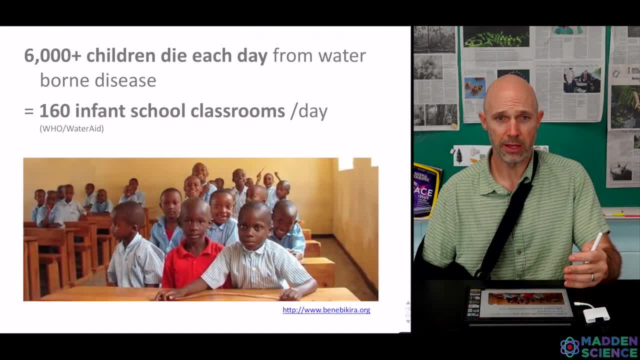 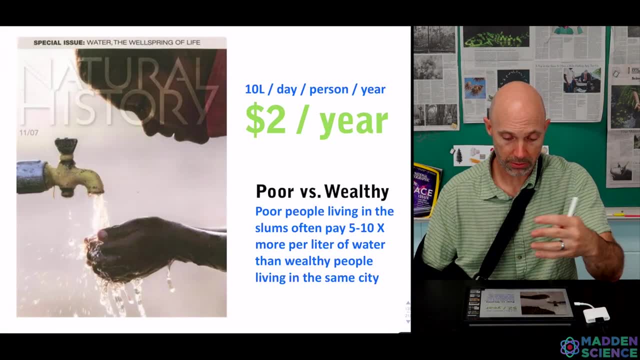 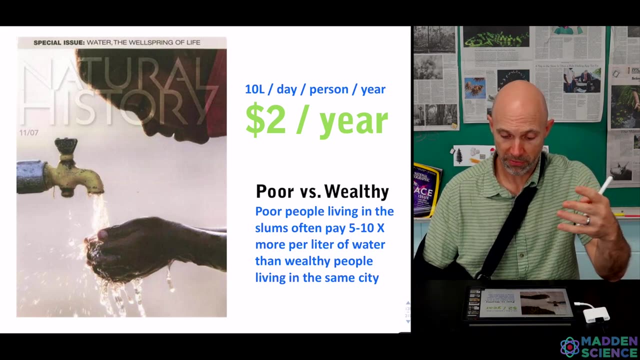 6,000 children each day, 160 infant school classrooms a day. One of the major killers is cholera. You just think in terms of our economic and ethical approach on this. it might work down to $2 a day to help fix this. 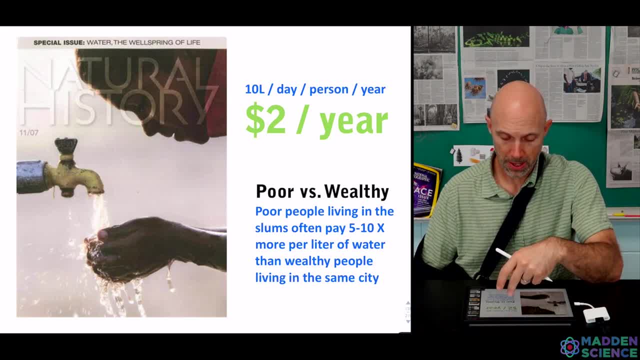 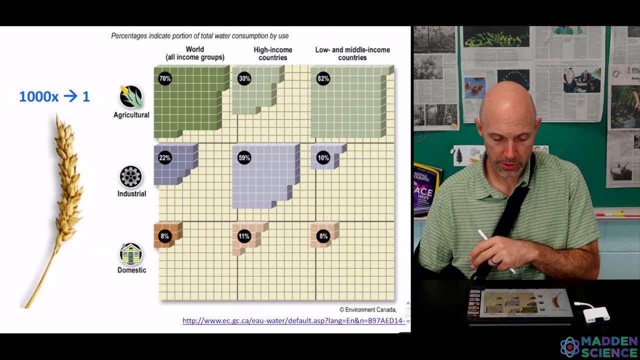 Another ethical and political component is that poor people living in slums often pay significantly more for their fresh water. In terms of water use, just quickly, this will come up more later in the year, but I want to throw it in just for some figures. 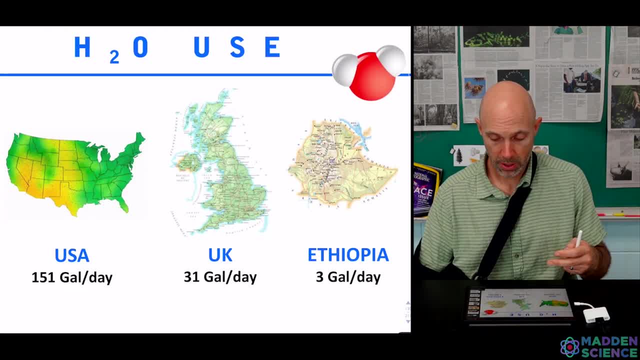 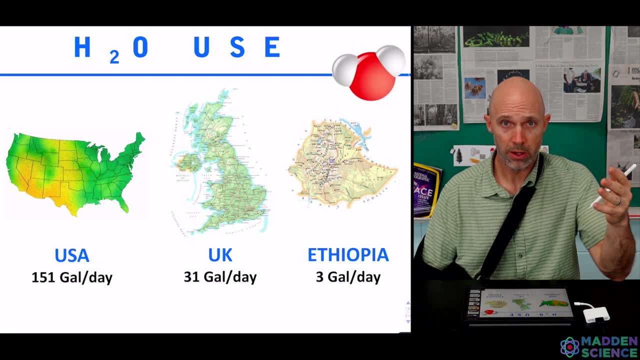 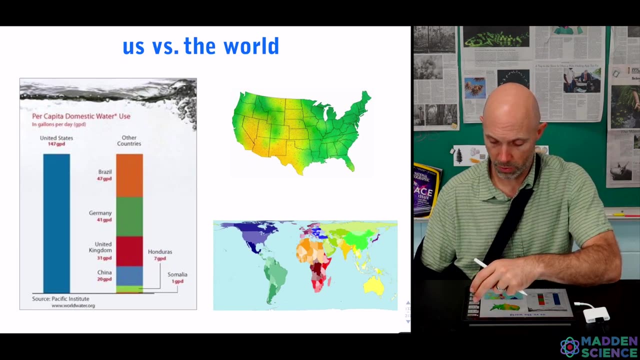 Water use in the US versus UK, versus Ethiopia pretty stark. We could even do our water footprint. that would then compare or relate to earlier when we did our ecological footprint. Here it is for showers. We got US versus the world. 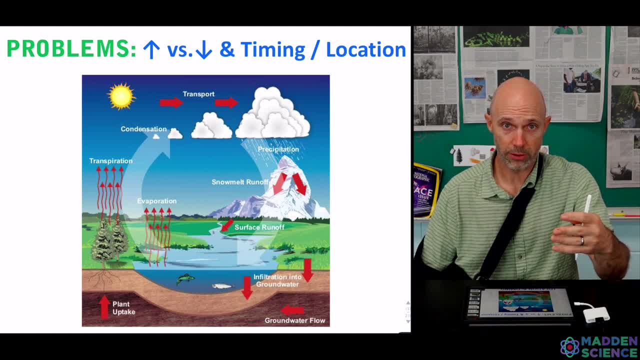 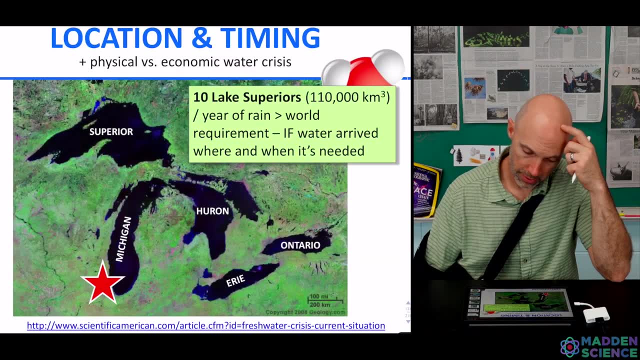 Again the problems within the water hydrologic cycle, not just with how much, but when and where the water is falling. Just a number for you: You got 110,000.. 1,000 kilometers cubed fall in a year. 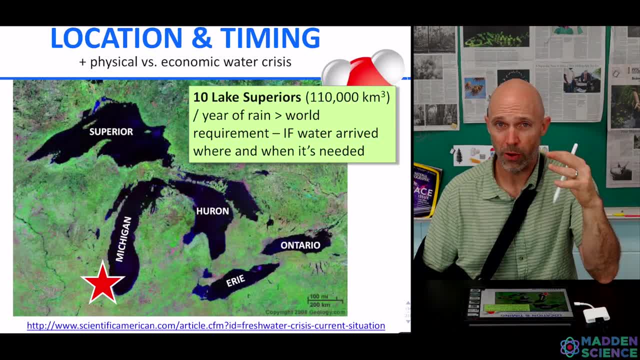 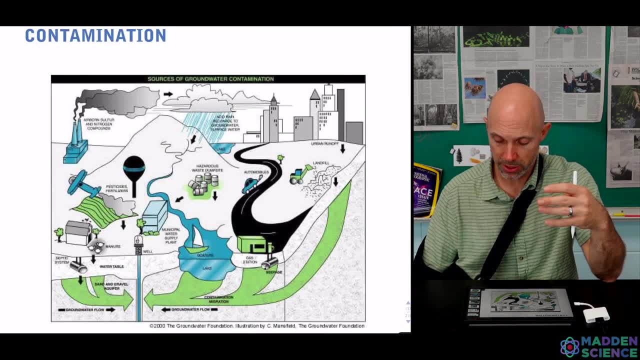 That's like 10 Lake Superiors, But as you notice in the news, it's falling unevenly and at the wrong time in many cases. In addition, there's contamination issues and problems. This ties back to our ecosystem services and the importance of that. 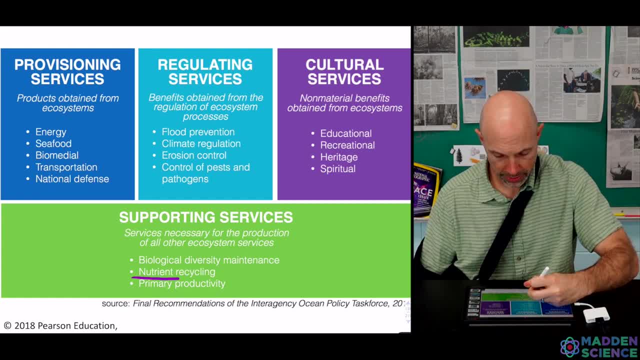 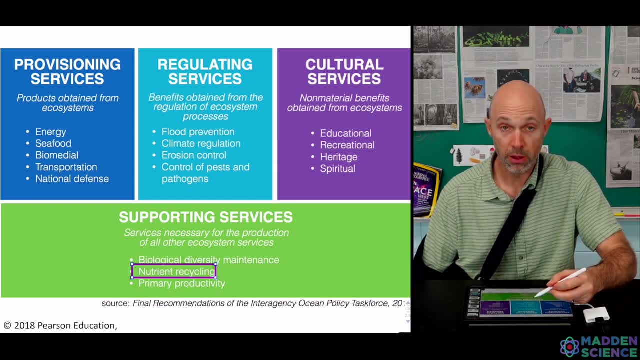 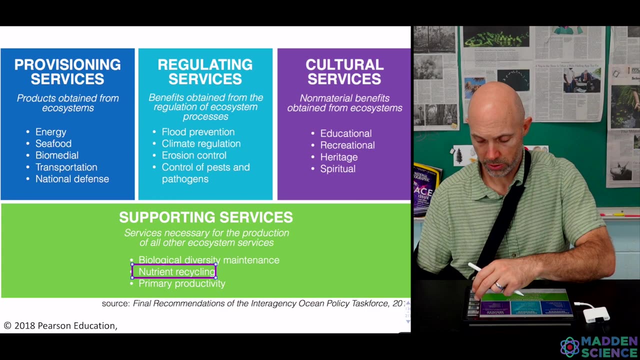 If you look at this, we've got nutrients recycling down here, which is tying into a number of things including climate regulation, flood prevention, pests and pathogens, transportation, seafood, energy, you name it. Here's another visual showing those supporting and provisioning and regulating services. 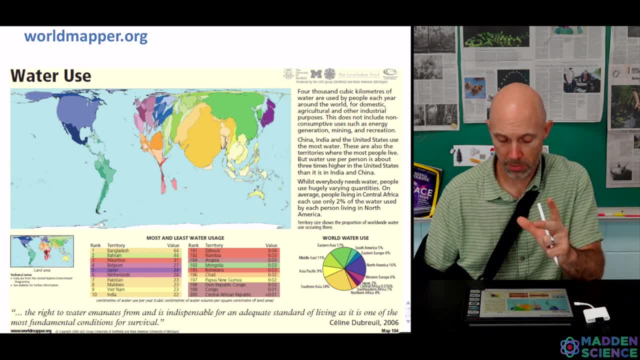 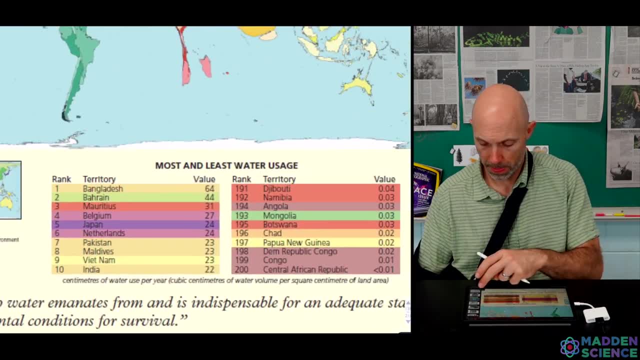 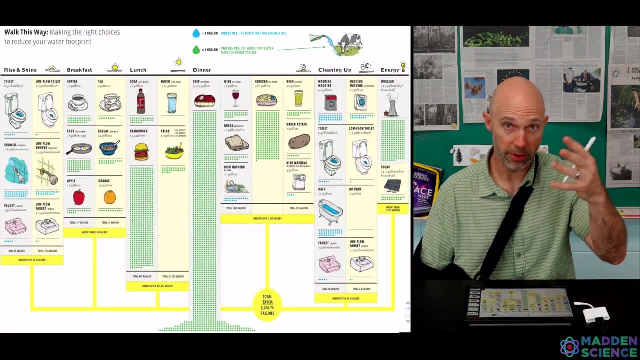 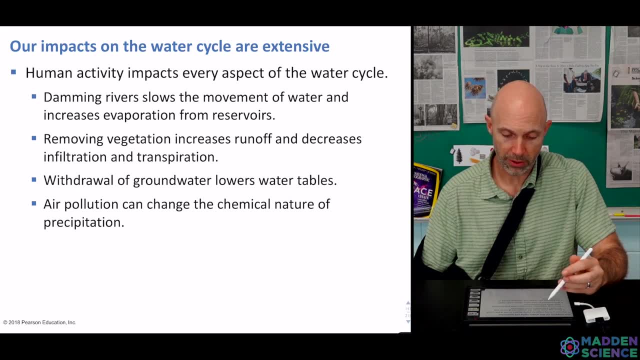 And then our water footprints look like. so The amount of water that it takes to produce different things. You can pause and zoom in on some of those Generally from the book. impacts on the water cycle are extensive: Damming rivers, runoff from removed vegetation, groundwater being lost. 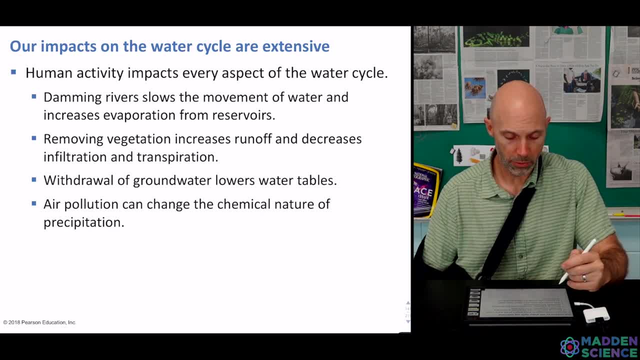 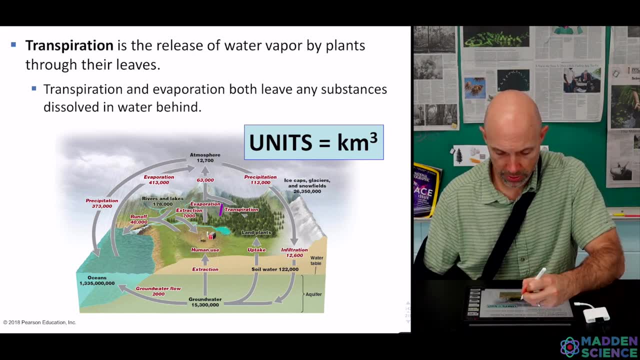 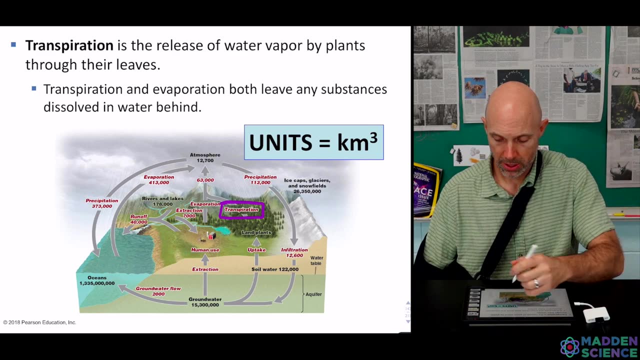 See that with the Ogallala Aquifer in the Middle West and the United States. So back to this. You can highlight different parts. This slide shows Transition. Transpiration is the part of flux as water exits plants. Remember that from biology. 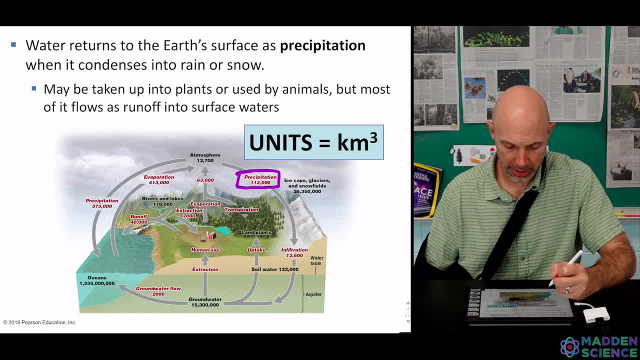 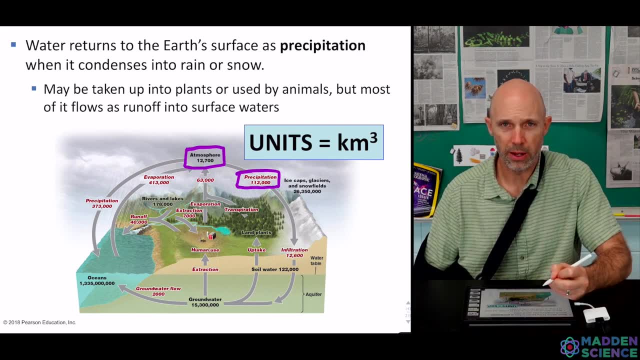 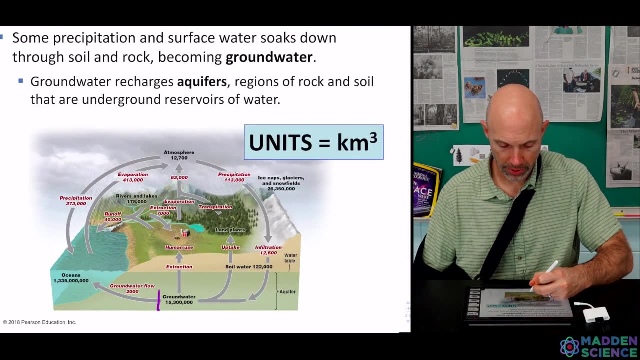 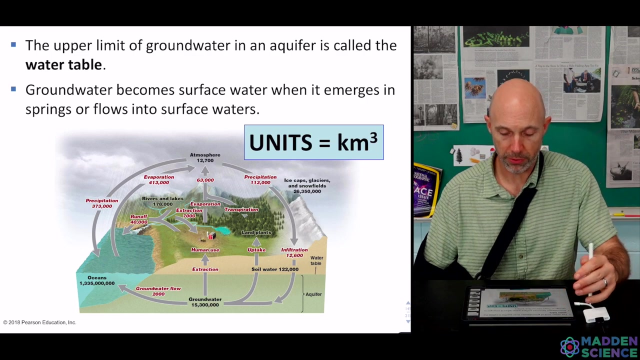 This is shown with precipitation coming in 113,000.. Earlier we were looking at atmosphere, so I think that number was correct at 12,700.. You can also see for groundwater. we mentioned with aquifers and additionally the water table. so how much water is in that aquifer? Now back. 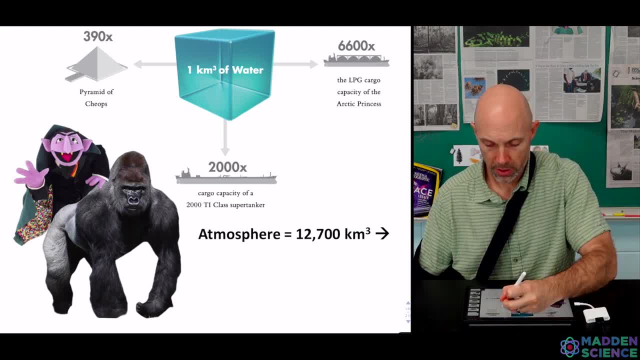 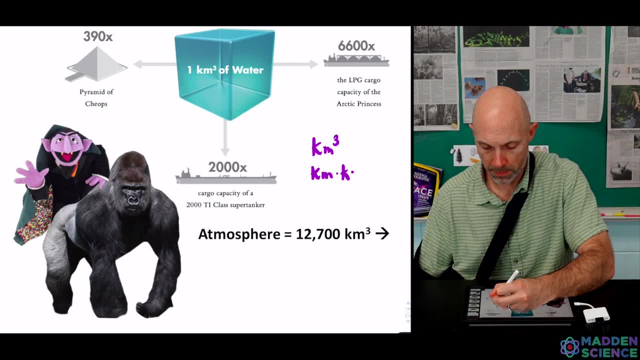 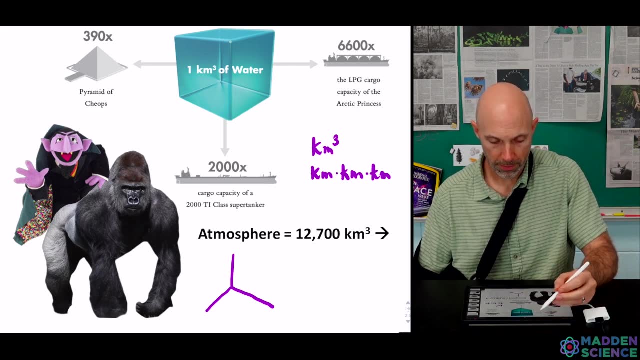 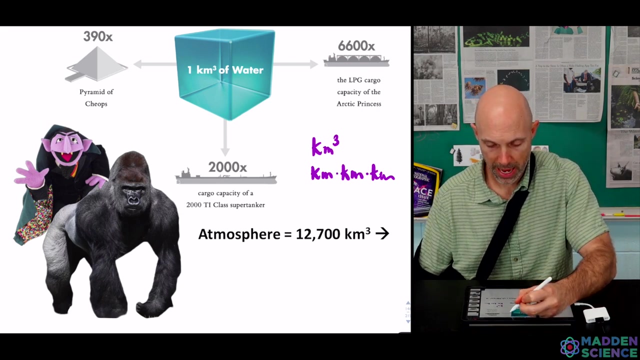 to our unit, which is kilometer cubed, so that's a kilometer times a kilometer times a kilometer. so you can imagine looking at it, you know, in three directions or, as we have this box here, you know each side is one kilometer. you. 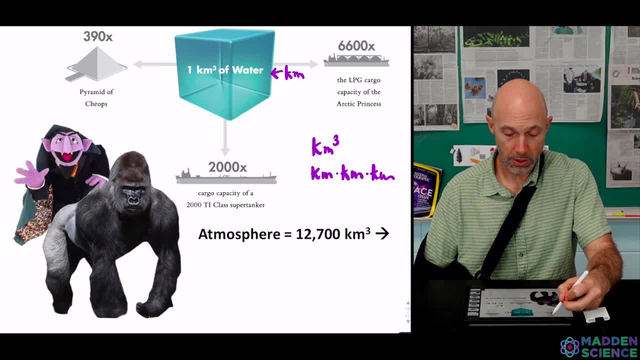 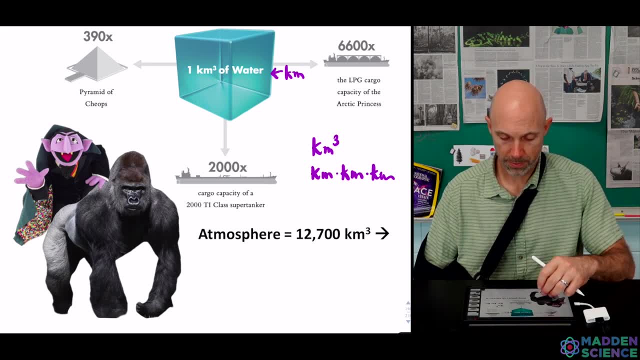 can do this with meter sticks to see. but yeah, this amount of water would be 390 times the volume of this pyramid, 2,000 times the cargo of one of these massive tankers. so you could, if you wanted, convert twelve thousand seven hundred hundred tons of water and convert it to a million tons of water. 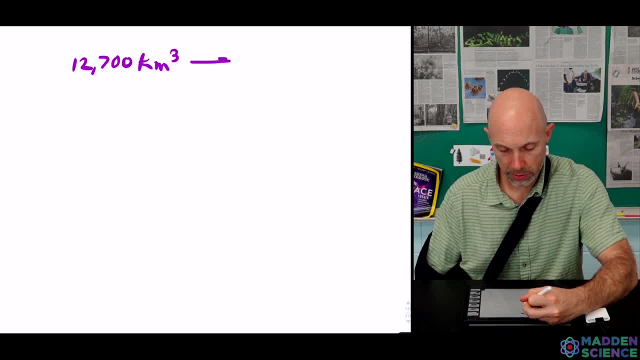 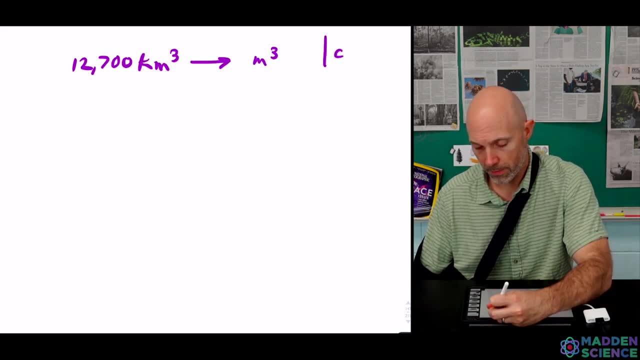 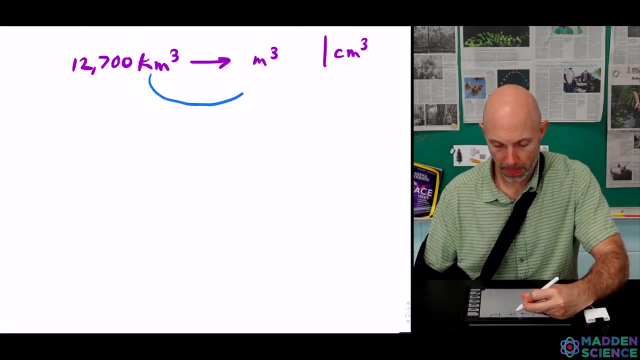 kilometers cubed into cubic meters or perhaps cubic centimeters that you could do later. what you want to realize is that the conversion between kilometers and meters is that there is one kilometer and a thousand meters, so that will work, taking note that this is cubed, so we'd have to do a three thousand. 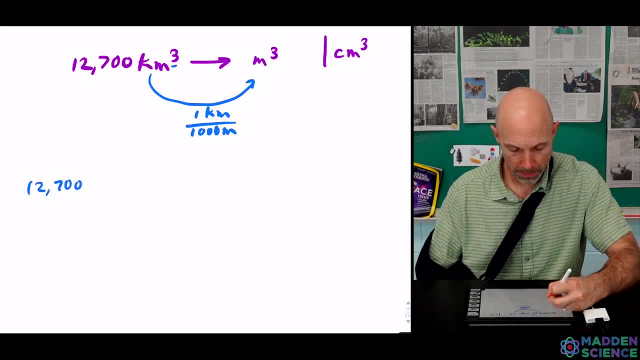 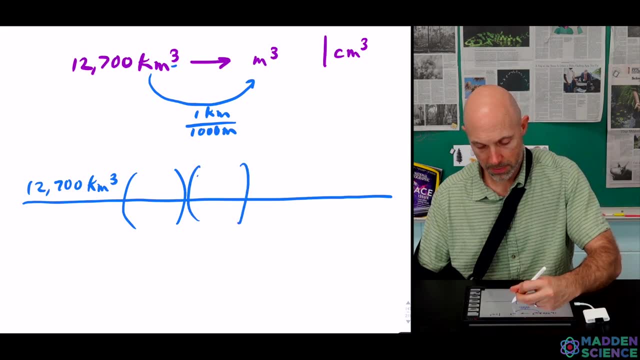 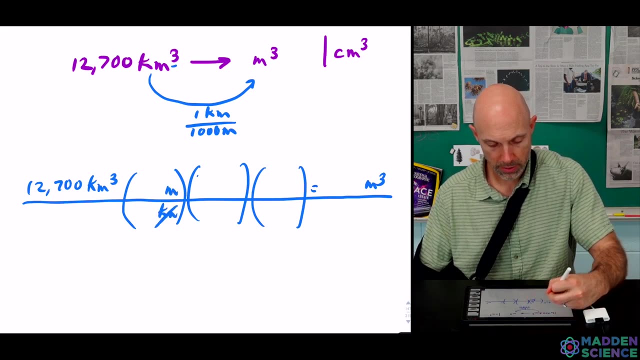 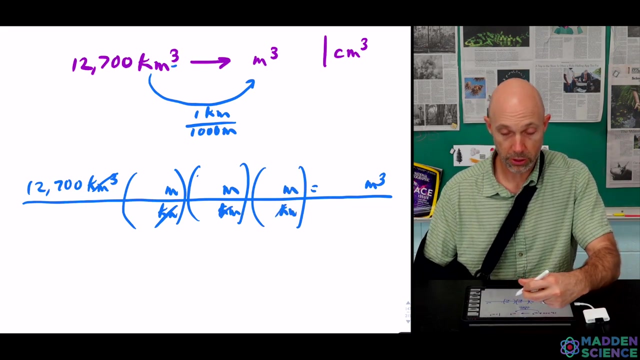 three times. here's our conversion: so we could roll out and do it three times to get two meters cubed and where we'd have meters, kilometers, meters, kilometers, meters, kilometers, where the kilometers cubed would cancel on the bottom and end up with meters on the top. so a thousand kilometers. 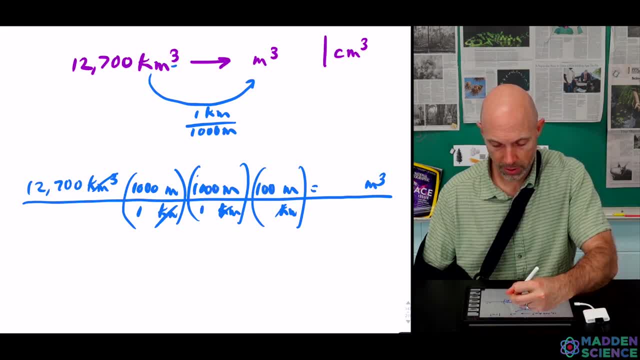 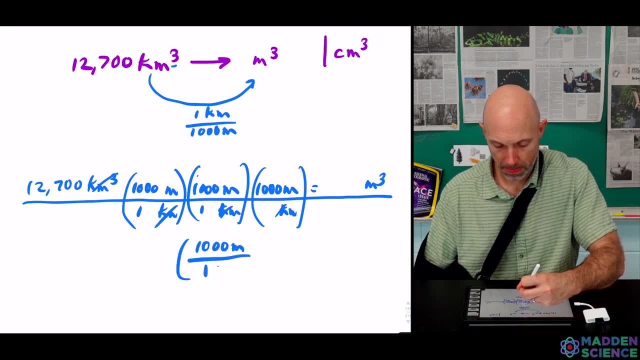 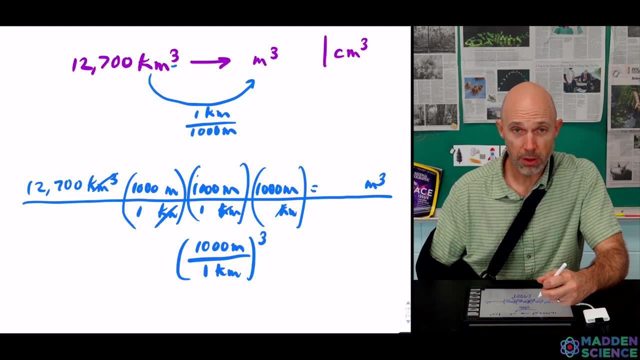 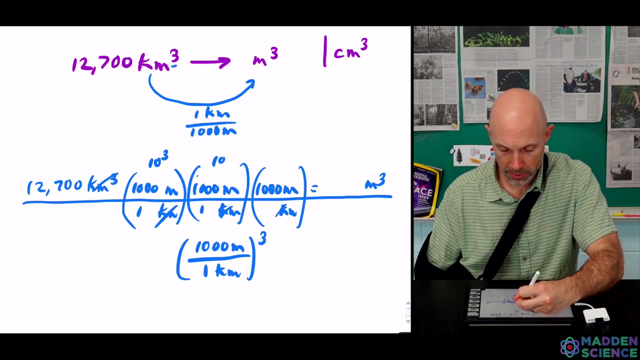 over one thousand, over one thousand over one, or combine those guys and just leave it as one whole thing cubed. if you do that, that's gonna be ten to the one, two, three times three times three, so it's ten to the ninth. combined that's going to be. 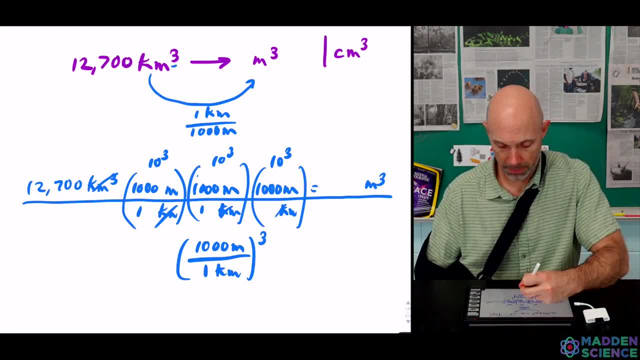 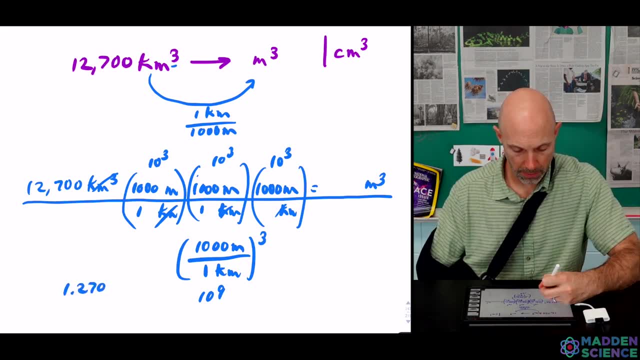 10 to the one, two, three times three times three, so that's 10 to the ninth combined here. Over here we can scientific notation: I'd put 1.270 times 10 to the 1,, 2,, 3,, 4,. 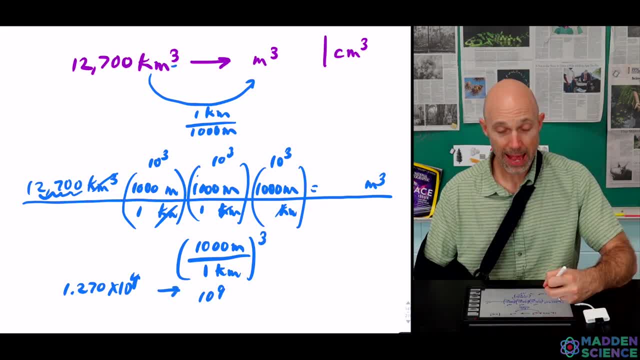 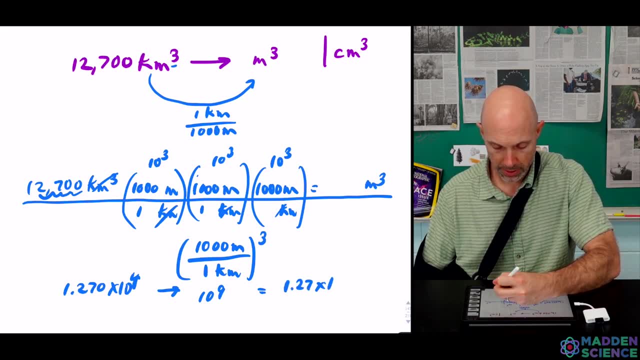 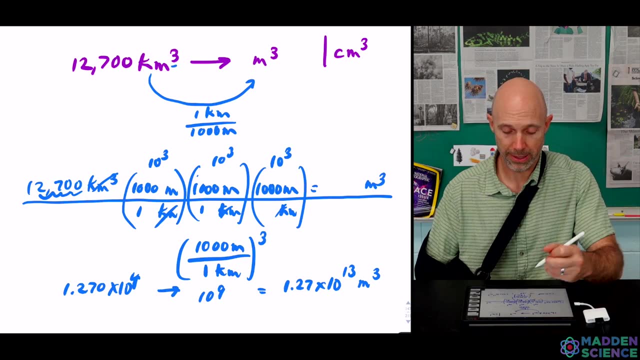 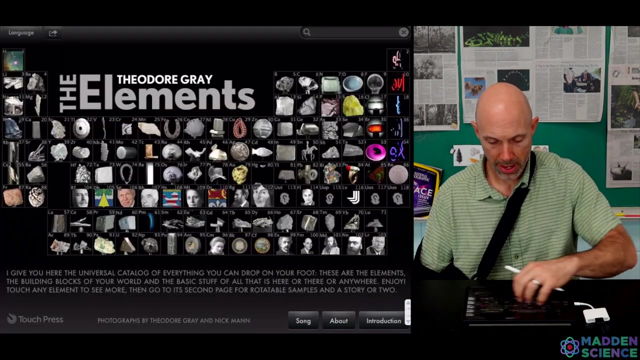 which means that your final answer for up here would be 1.27 times 10 to the 13th meters cubed. So that's a pretty incredible number if you write that all the way out, Moving on to carbon. So again we can look at our elements over here. So we started with water. 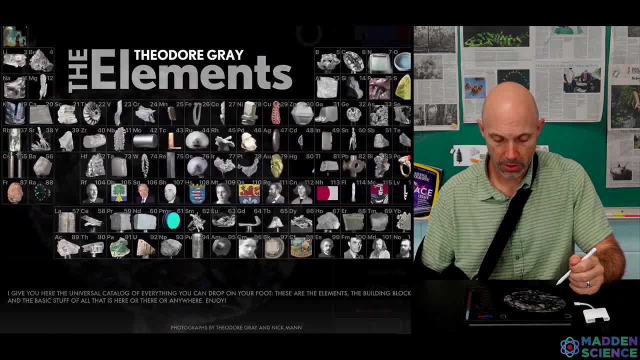 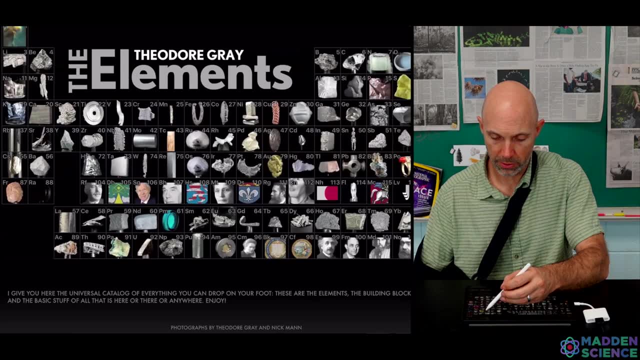 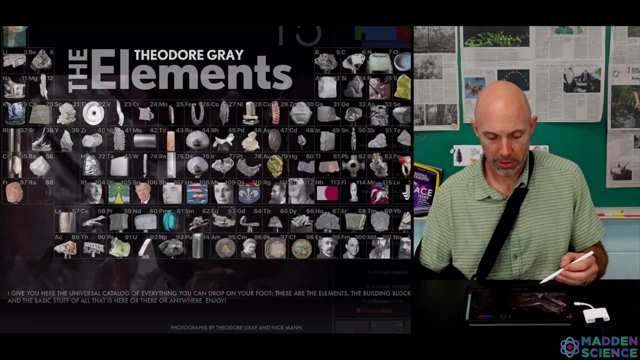 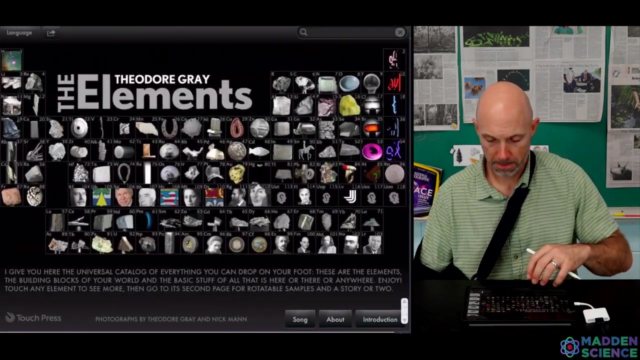 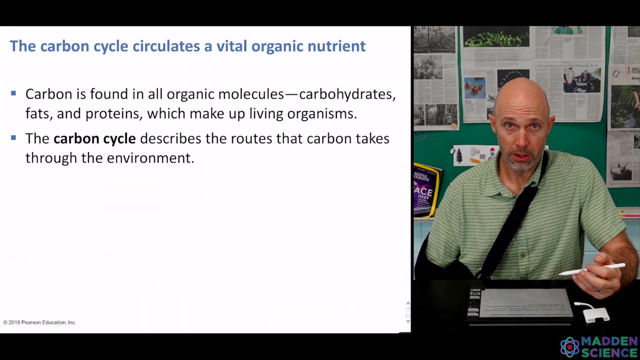 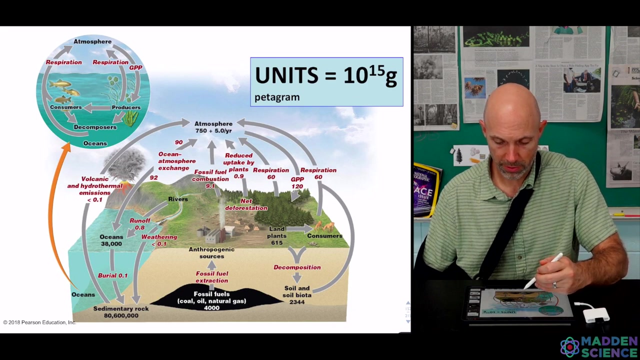 as a molecule. Now we're into carbon. We'll get into nitrogen And end with carbon And end with phosphorus. Here's carbon, Carbon and its cycle, most important and most related to talking about climate change these days. Here it is where these units are, in fact, in petagrams, or 10 to the 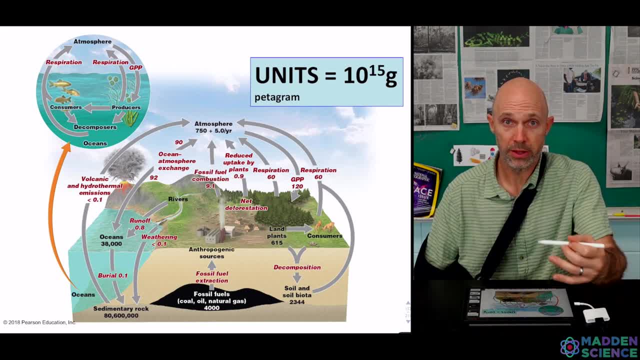 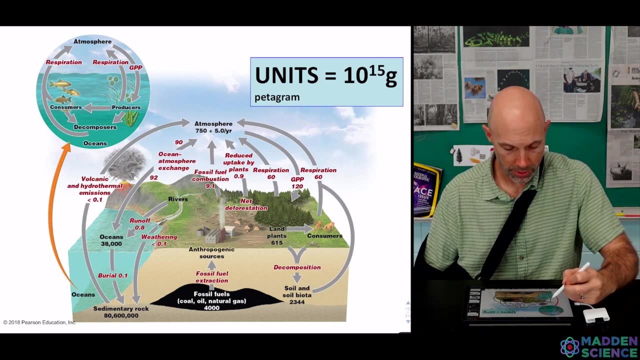 15th, So that's 1,000 times more than a teragram. So you're hearing about terabytes these days, which are 1,000 gigabytes. So you're going in there a kilo mega and all the way up to peta, which is 10 to the 15th. So a lot. 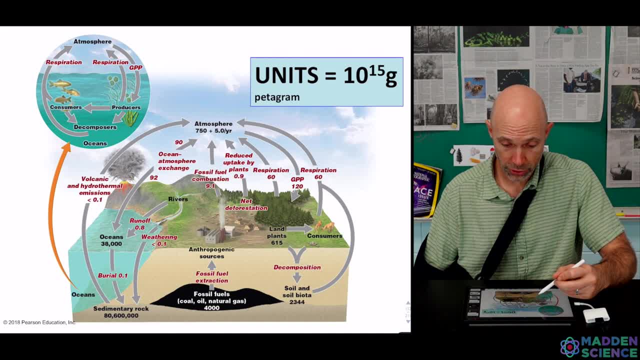 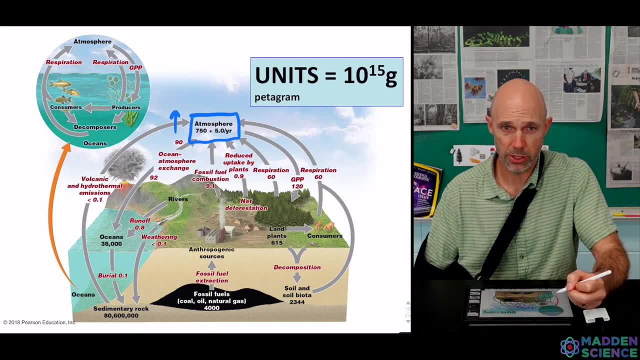 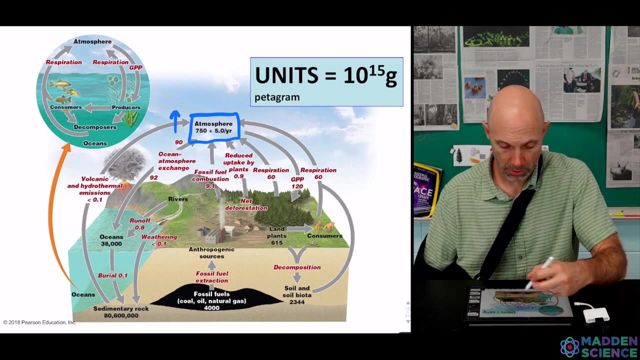 of flux. Again, this is going to be seasonal, certainly changing. One of the major things that is changing is the amount of atmospheric carbon dioxide, which is going up. The ability of certain lands to serve as a reservoir may be decreased. So again, just take a peak, Maybe in Paul's video. look at some of these numbers. One: 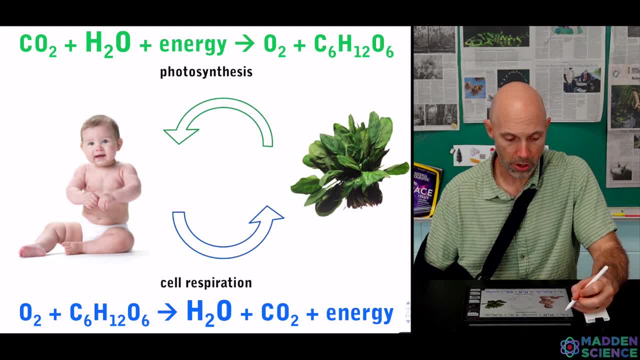 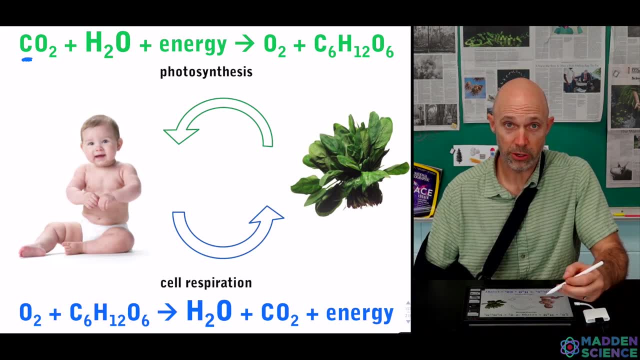 of the major drivers again is that exchange of carbon, Carbon dioxide- that essentially gets fixed by algae, some bacteria in plants via photosynthesis, and then production of carbon via cell respiration. So this combustion of sugar is similar to what you'd find via 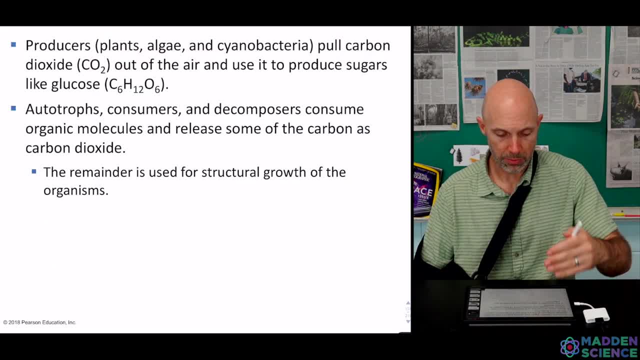 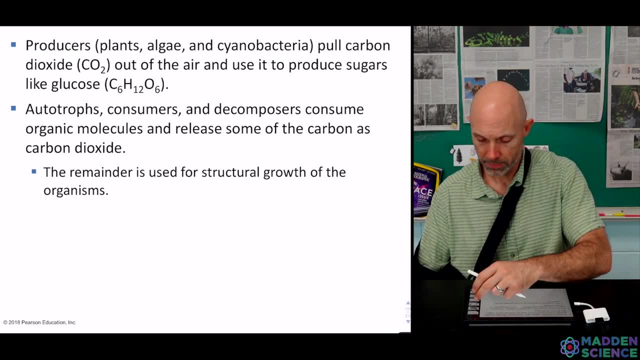 car or a power plant. so keep that in mind Again. producers right: plants algae, which would be protists, cyanobacteria, fixing that carbon. Little bit more in terms of this, you got aquatic organisms and that recycling. 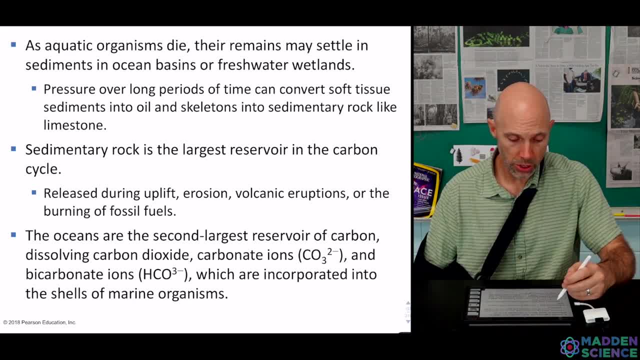 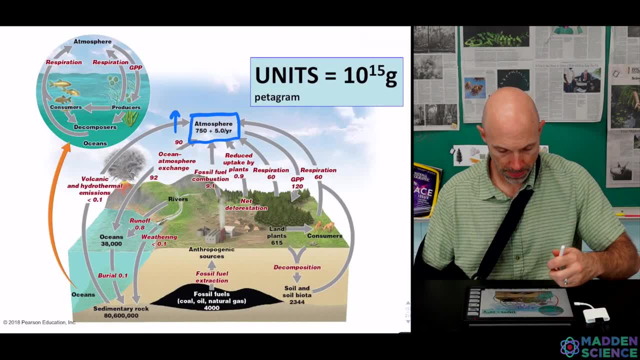 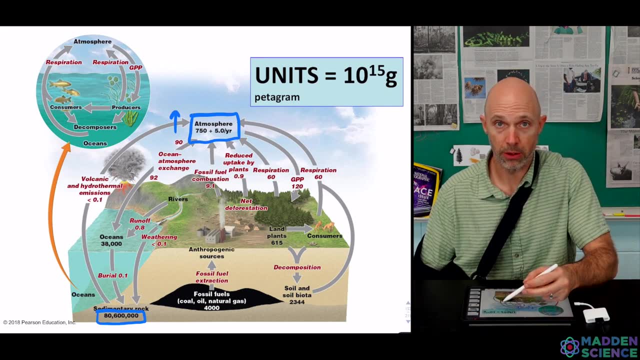 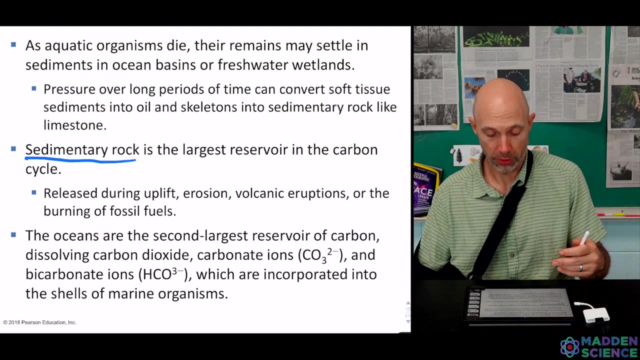 right forming fossil fuels, huge reservoir in sedimentary rock. So if we go back here you can see 80 million times 10 to the 15 grams of carbon stored there, Ocean being the second largest reservoir. so this'll tie in later when we get to ocean acidification. 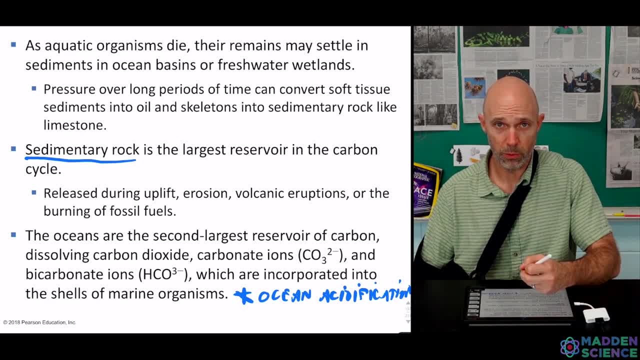 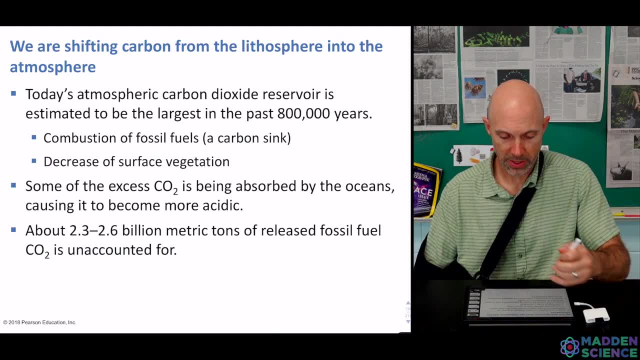 which ties into yesterday's talk when we dealt with water and pH. A few more ideas in here. Today's atmospheric carbon dioxide reservoir is estimated to be the largest in the past 800,000 years. So again, that's the amount of CO2 in the air. 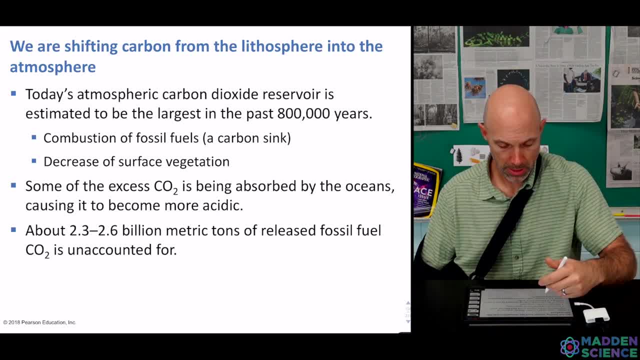 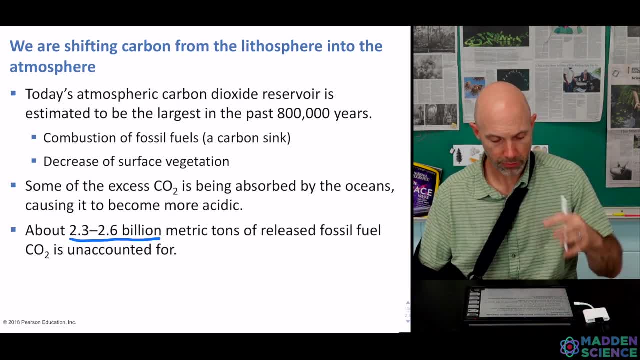 So oftentimes. in parts per million, You can see that 2.3 to 2.6 billion metric tons released fossil fuel- CO2- is unaccounted for. so a little bit of flux in there. Moving on to nitrogen, another beautiful and interesting. 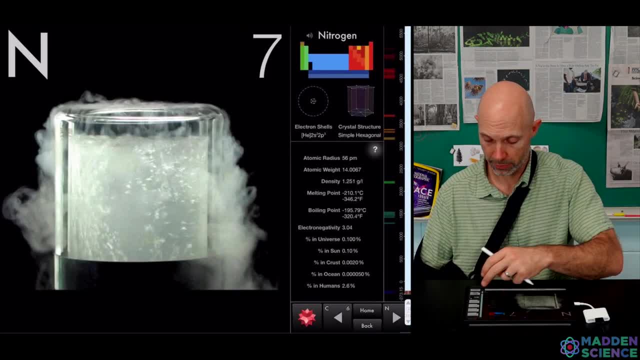 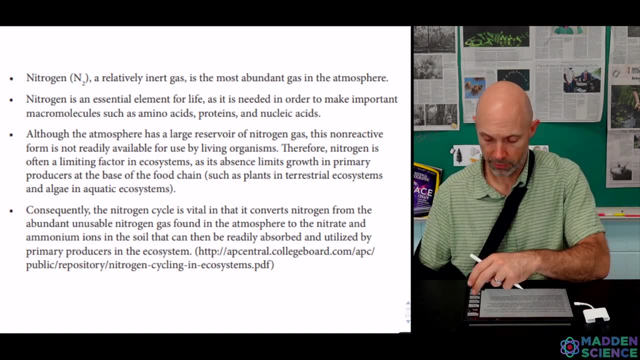 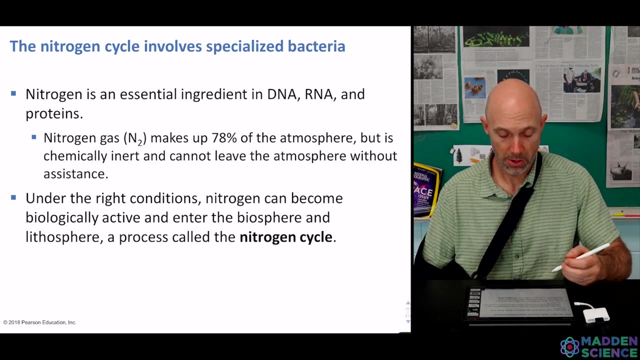 interesting element with a complex and intricate cycle, Got our CED. We already showed you. this slide give you a little background on nitrogen, which you may recall from chemistry times. Nitrogen being essential, you got it as essential part of amino acids, right? 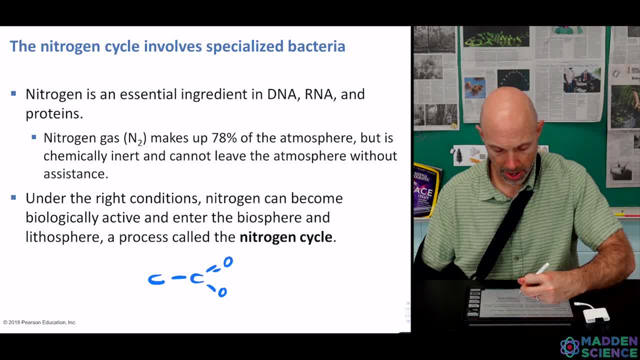 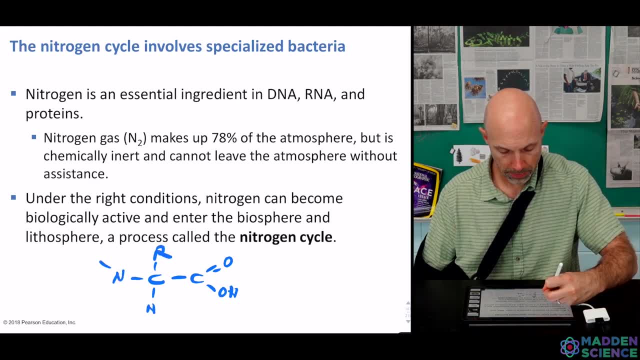 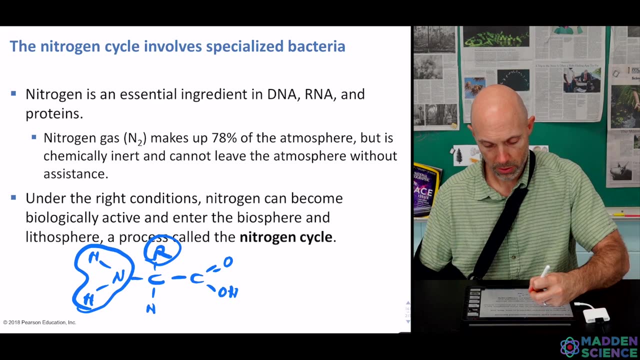 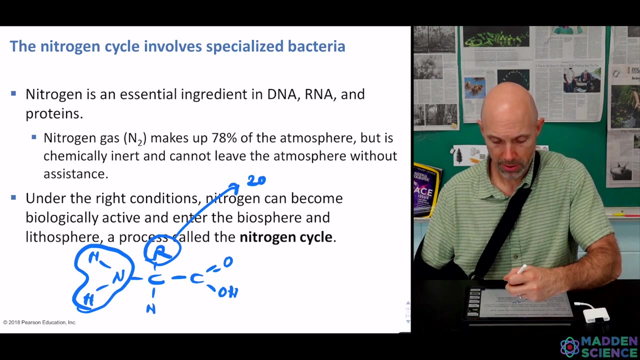 So you got your central carbon carboxyl group, your R group up here and then your amine group here. right, And recalling that there are 20 different R groups to make up the naturally occurring 20 amino acids. These guys come together via peptide bonds. 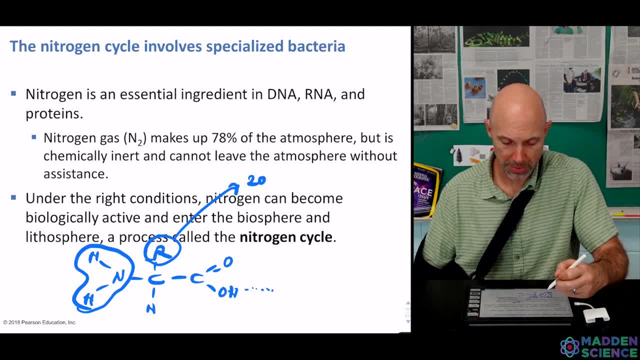 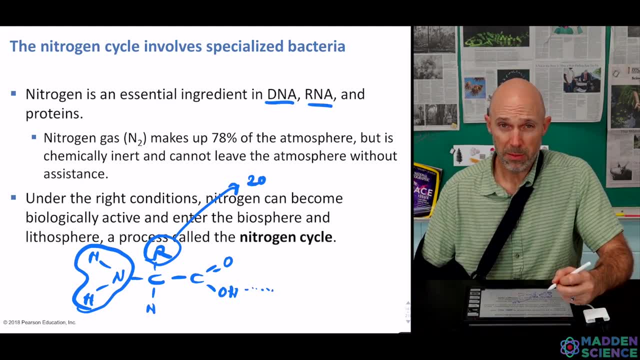 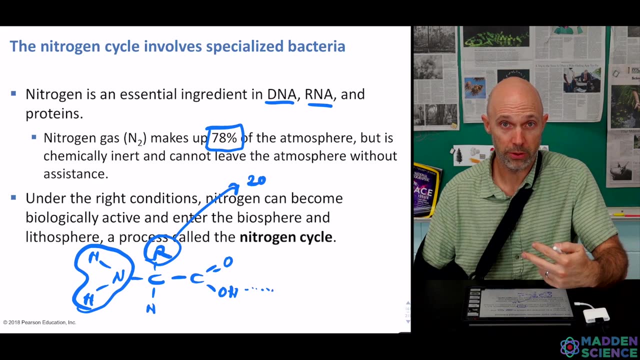 making up long chains of hundreds, perhaps thousands of amino acids. So although it's important in proteins- obviously DNA, RNA- it makes up a vast majority of the atmosphere And that's not usable, almost inert to us, So we have to rely on other organs that can fix it. 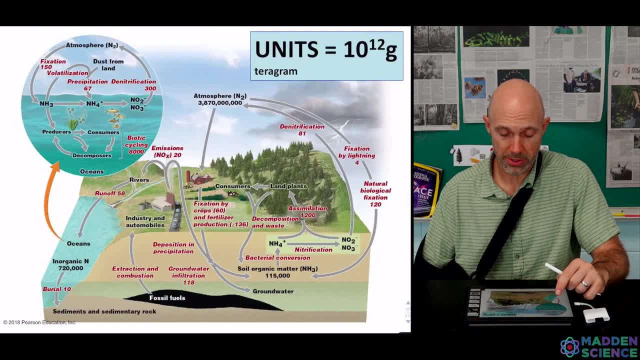 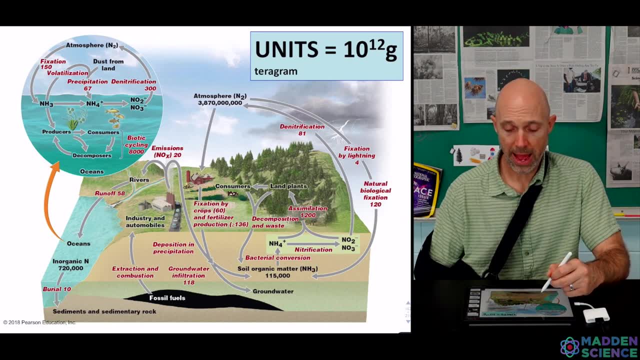 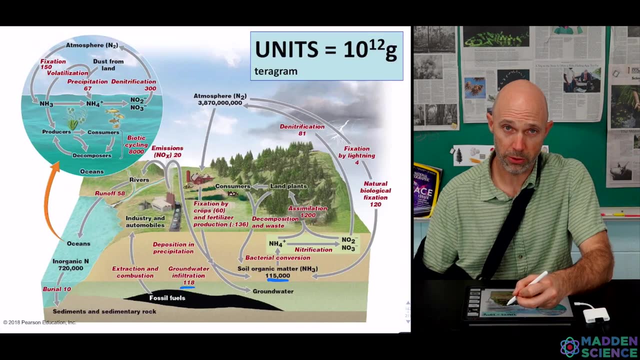 So put it into a usable form. Here's our nitrogen cycle. You can see both the aquatic and the terrestrial, or water and land, aspects of this. The units that you're seeing in here are coming in teragrams, or 10 to the 12th grams. 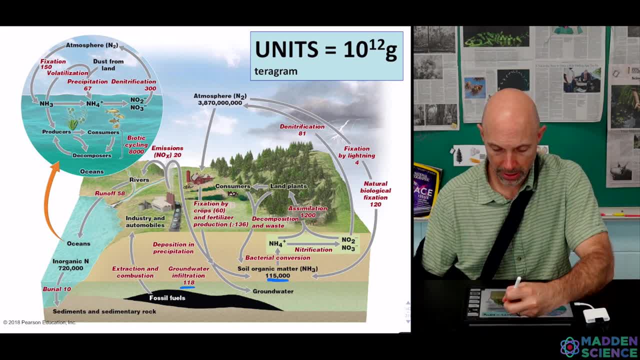 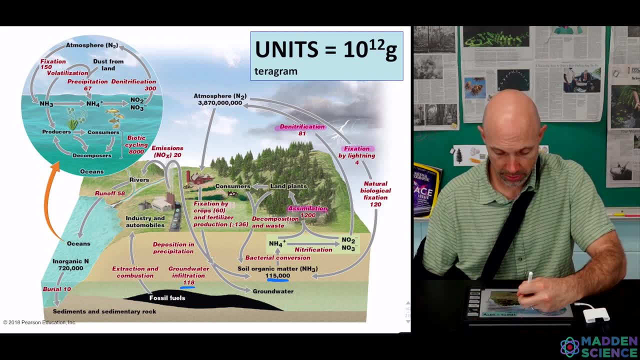 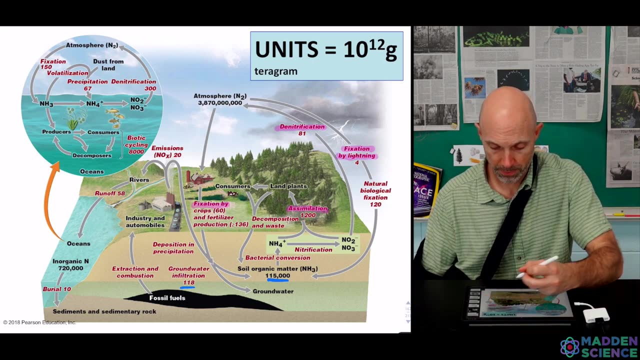 So highly complex. The most important parts in here are gonna be, at least for our purposes, denitrification, assimilation, fixation again by crops, and fertilizer by bacteria by some plants, by lightning The chemical transitions here with ammonium to nitrate and nitrites. 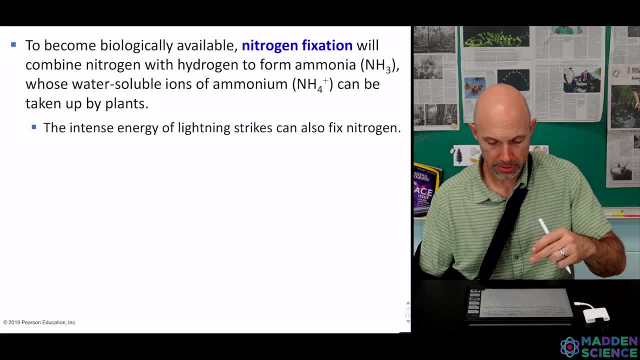 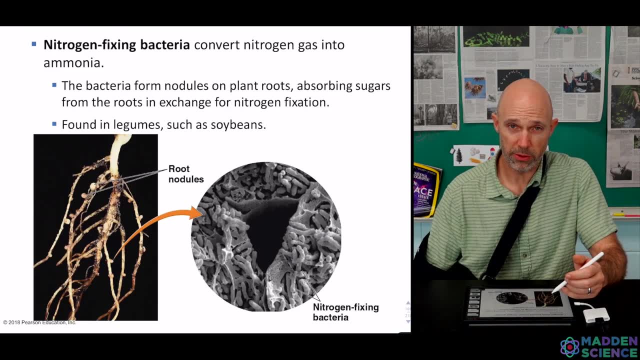 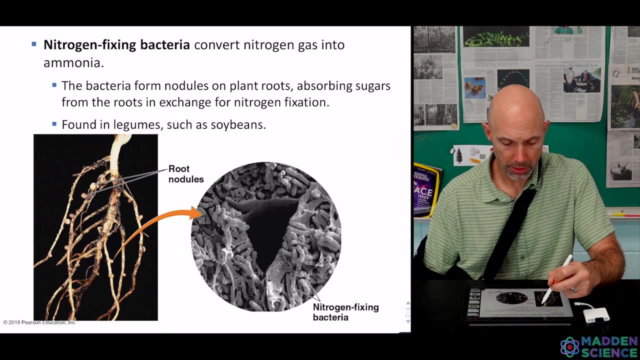 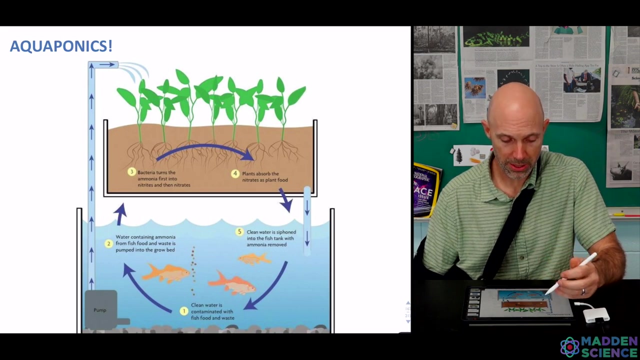 The way can be more payer-effective. You can see again. you can focus on the aspect of nitrogen fixation. This is gonna be essential with nitrogen fixing bacteria Also works here with roots. You have nitrogen-fixing bacteria here. Legumes such as soybeans are a good example of that. 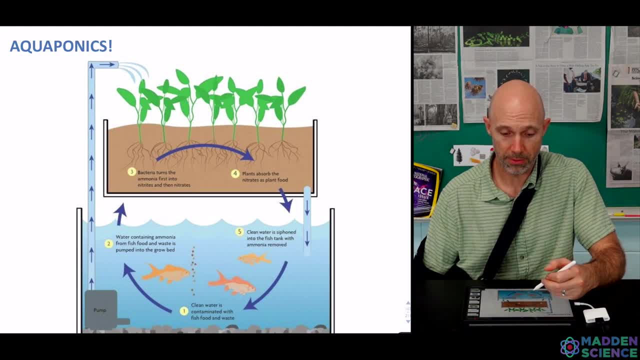 Good connection that I had with it, going back to the old days, was aquaponics other, where the fish down there urinate and they pee out ammonia and that gets filtered back over the plants and in the process you got naturally occurring nitrogen fixing bacteria, nitro back to bacteria, nitrosomonas bacteria. that 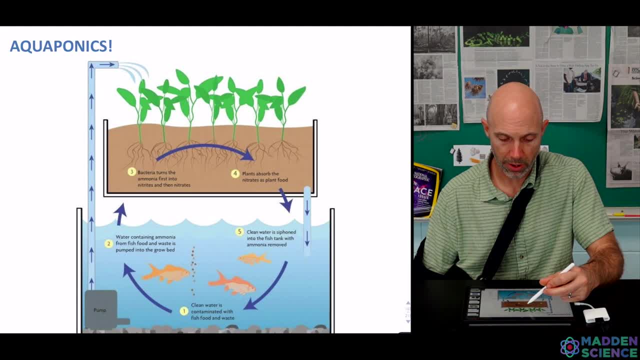 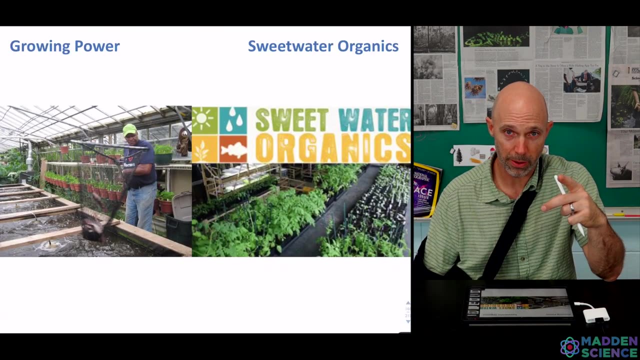 convert it into nitrites and nitrates and therefore act as fertilizer for the plants. so the plants, in the sense, essentially clean the water it comes back. so you have a closed system, kind of like what we're trying to do with our eco spheres. big shout out to my friends at growing power and Sweetwater. 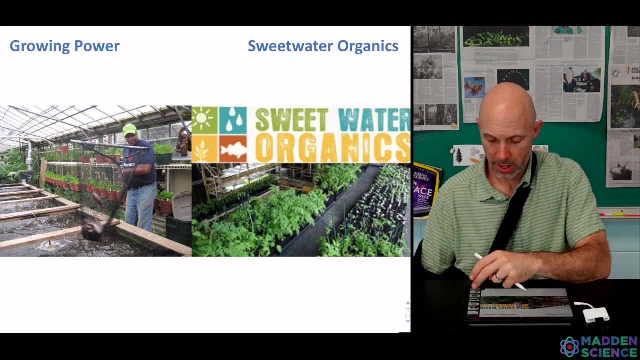 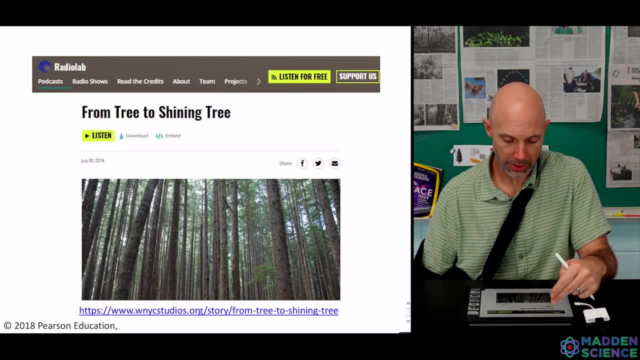 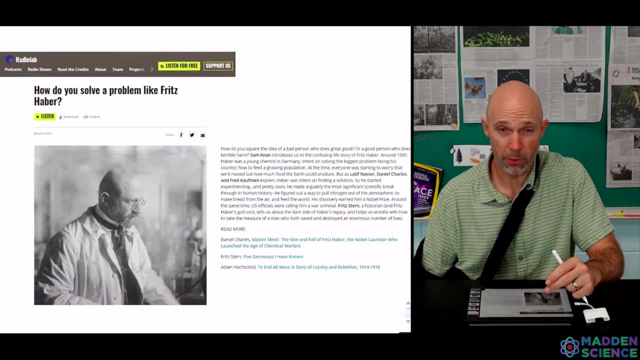 organics in Milwaukee for helping me out years ago. quick piece of info that I'm gonna put in the comments will be from tree to shining tree. a awesome radio lab about my core is a, and fungal networks another radio lab. that's really cool. it's on the. 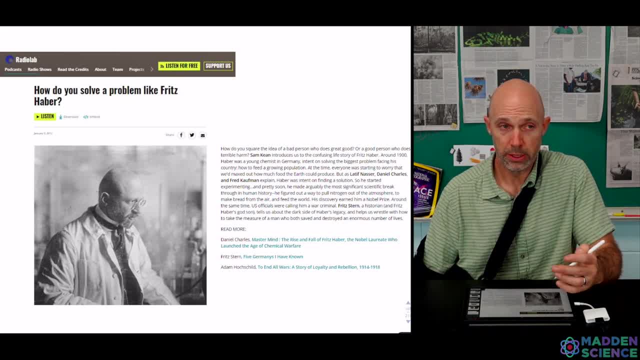 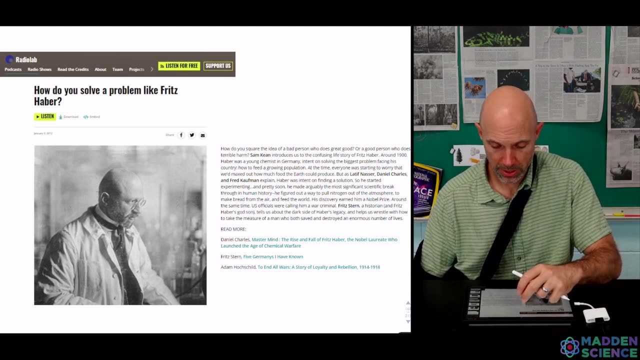 pad show kind about Fritz Haber who won a Nobel Prize, maybe had the greatest invention in the history of humanity: his ability to chemically in a lab fix nitrogen, to make nitrogen fertilizer to increase plant yields. you can read him about. read about him here. so around 1900 I was a young scientist, chemists, in 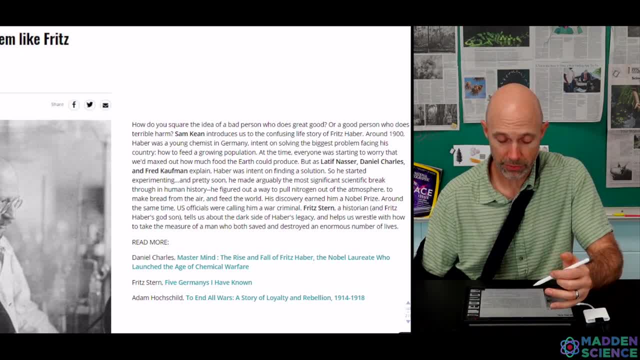 Germany and on solving the biggest problem facing this country: how to feed a growing population. so experimented pretty soon. arguably the most significant scientific breakthrough in human history- way to pull nitrogen out of the atmosphere- turns out. there was a dark side to Humber's legacy and how he wrestled with how to take the 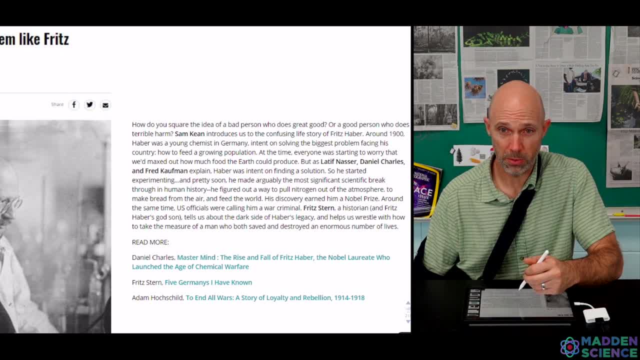 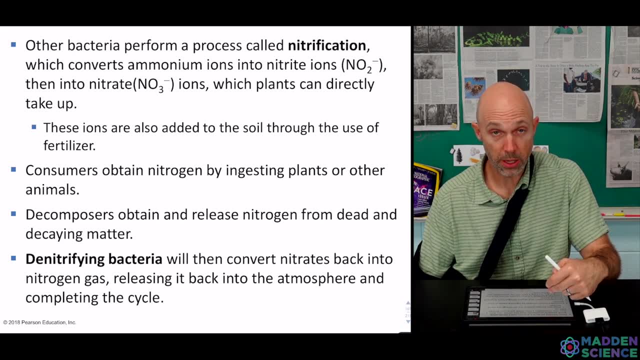 measure of man who both saved and destroyed enormous number of lives. so you can check that out. can go back through. yeah, consumers decomposers de-nitrifying bacteria back through. yeah, consumers decomposers denitrifying bacteria back through. yeah, consumers decomposers denitrifying bacteria. 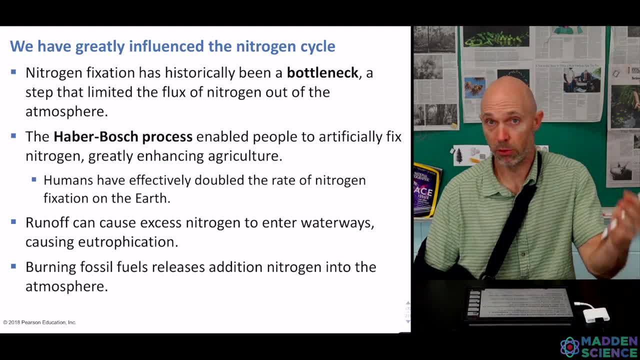 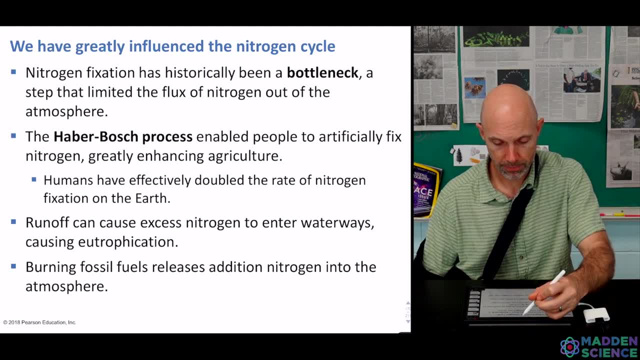 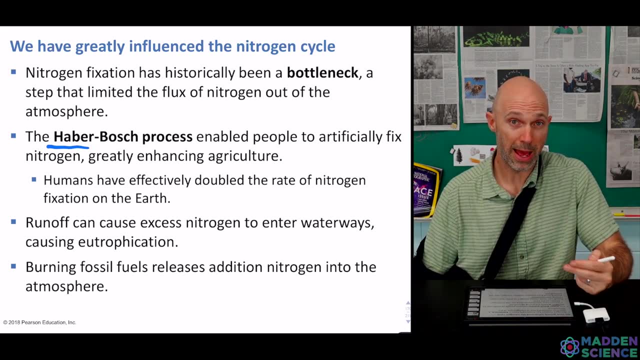 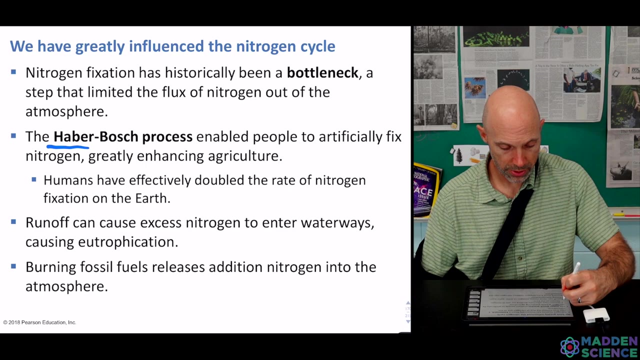 Nigerian fixation story was a bottleneck that limited the amount for the flux transition of nitrogen in its nutrient cycle can fit solder, and the hover Bosch process enabled us to artificially pull. makes good atmosphere can, too, too, useful form. this now has led to a number of other issues we've talked about already. 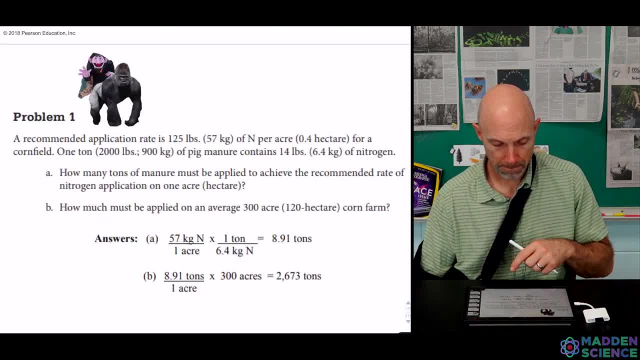 including water quality and water management, environment and the other two issues that we talked about already, including water quality and water distribution, and the other two issues that we talked about already, including water quality and water quality and runoff. Hey, some more apes math. So here's problem one: Check this guy out. 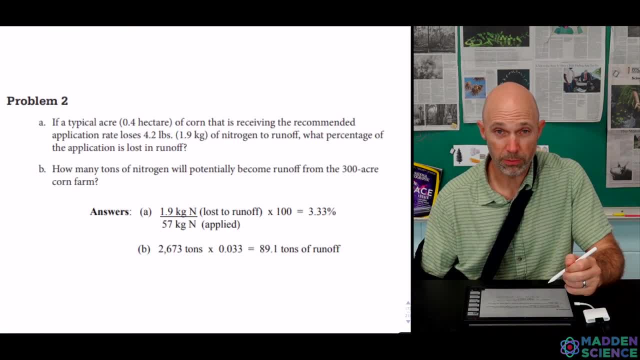 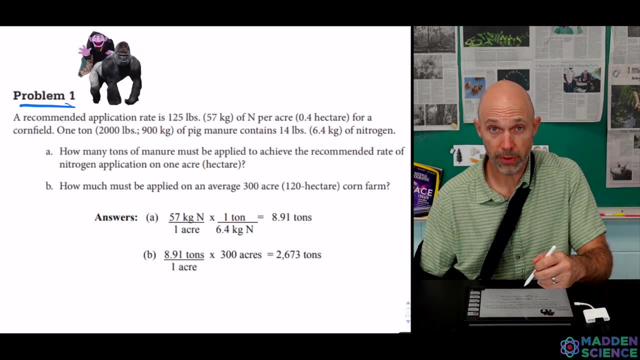 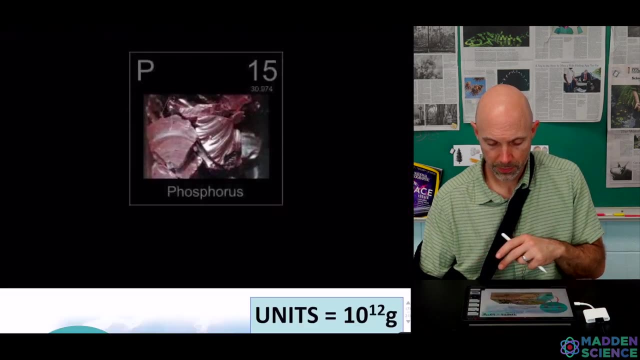 at home. And problem two, Check this guy out at home- Gets us to work a little bit on dimensional analysis and conversion factors, So think through it carefully. Moving on to our last guy, Phosphorus. Shown here It's cycle probably a little bit simplified from nitrogen or carbon. 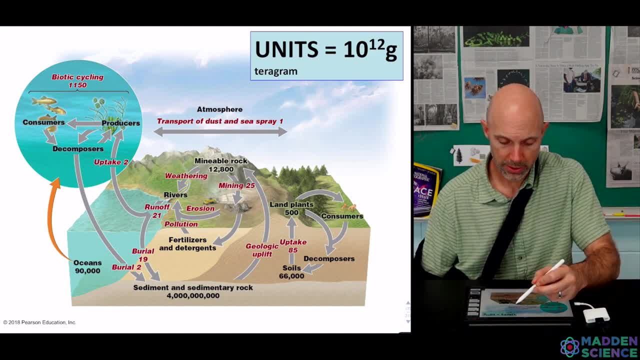 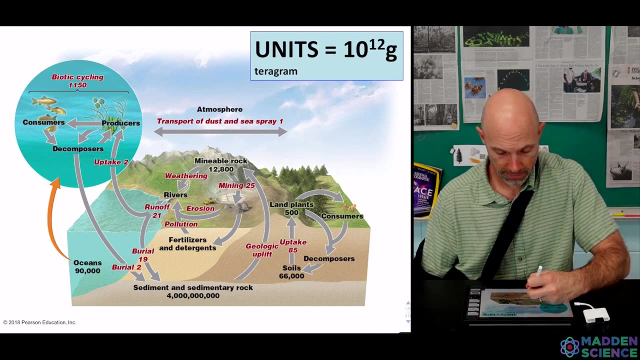 Certainly less talked about. Units in this are in teragrams. You can see once again reservoirs in black, Fluxes in red. They also have a significant aquatic or marine component. Notice, Ken, if you just look at the numbers, the vast majority is stored up in sediment, sedimentary. 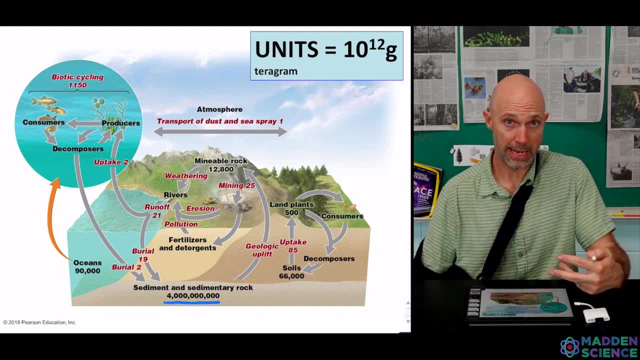 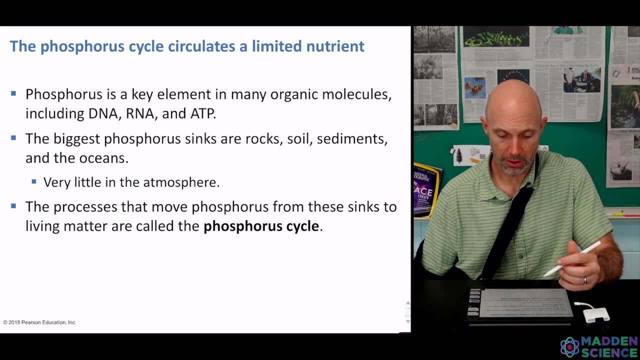 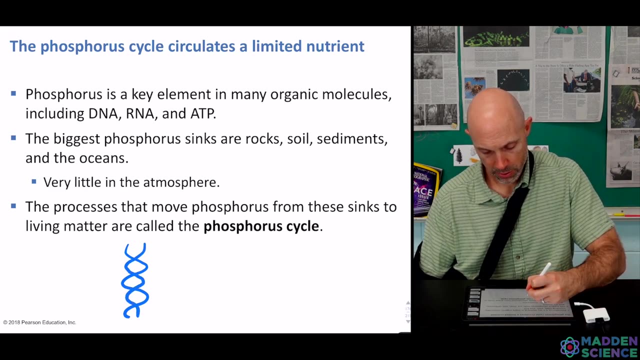 rock. We're getting this through the soil, through plants that we eat. So these are some of the nutrients we get from our food. Phosphorus: Right, if you look at the backbone of DNA and there's a sugar phosphate backbone, so that phosphorus within phosphate. 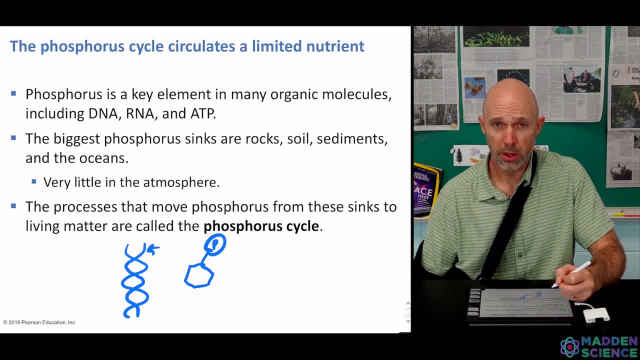 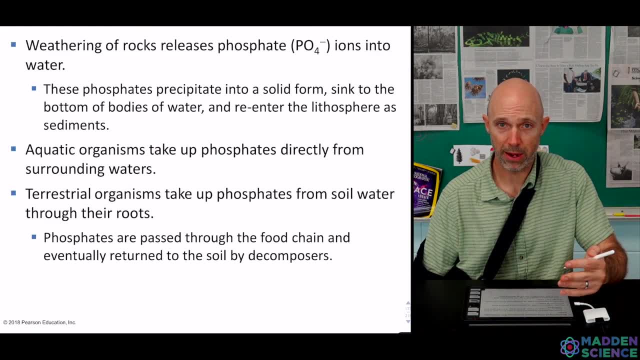 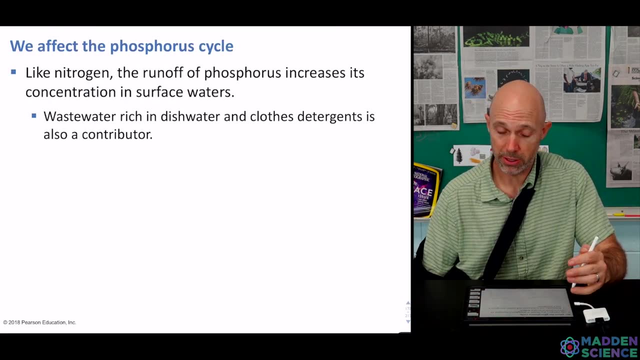 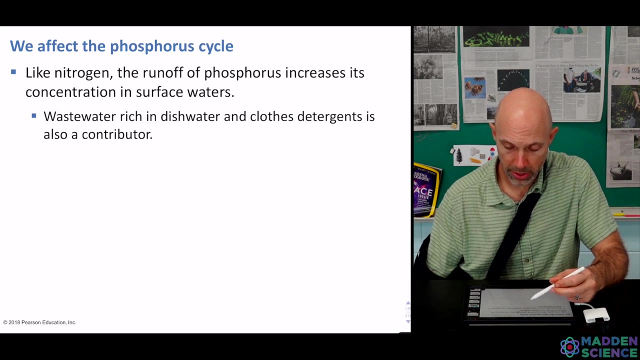 gum, essential as part of the sides or the backbone of DNA. We can see it released off of weathering rocks in the form of phosphate ions Like nitrogen. phosphorus runoff increases its concentration in surface waters. wastewater rich in dishwater clothes detergent is also a contributor, So you might see both of. 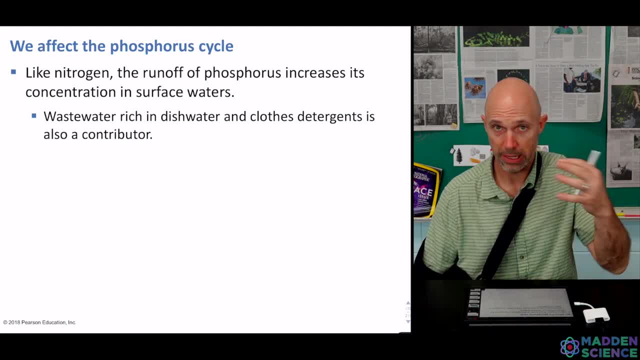 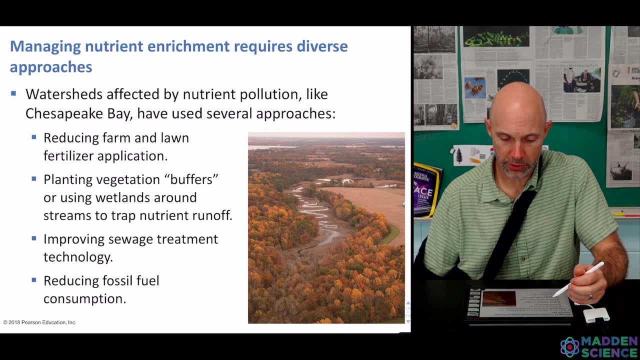 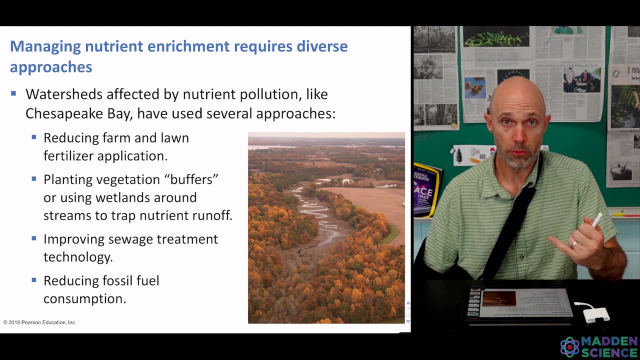 those things for clothes and your dishwasher detergents, say, like low phosphates. This section closes out with managing nutrient enrichment and realizing that it requires a whole lot, as things are changing and we are impacting the reservoirs and fluxes of these systems. So here's a number of 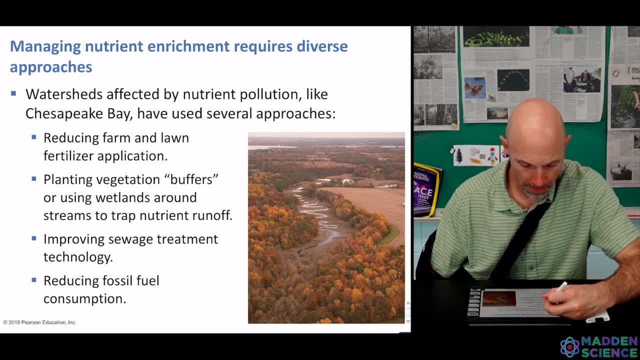 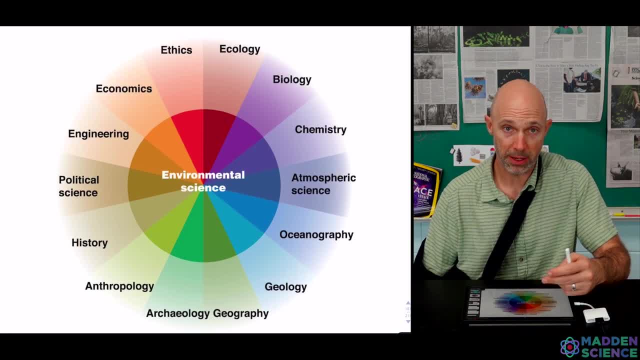 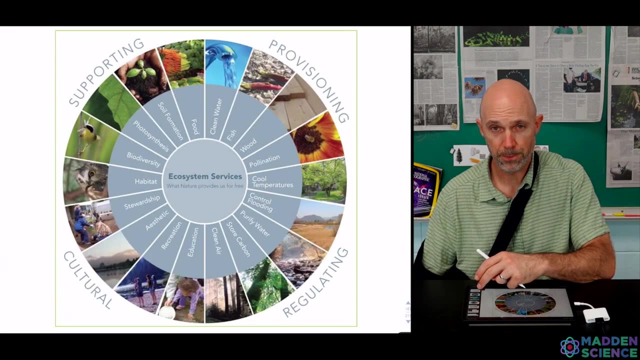 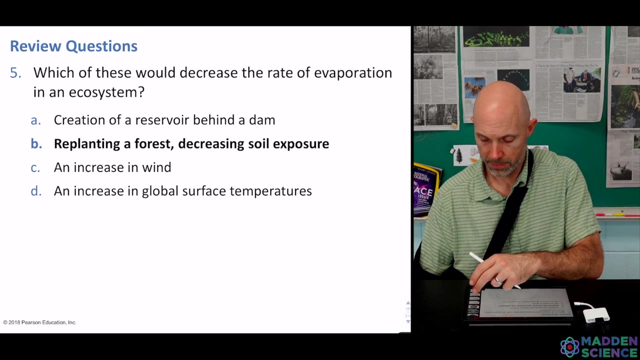 options, including ones in the Chesapeake Bay, Gives us some of the costs, which relates back to, clearly, economics and ethics, and also rounds us back to ecosystem services shown here. Alright, that wraps it up. Check out our OneDrive for some of the questions on here. You can see at the end there are just two. 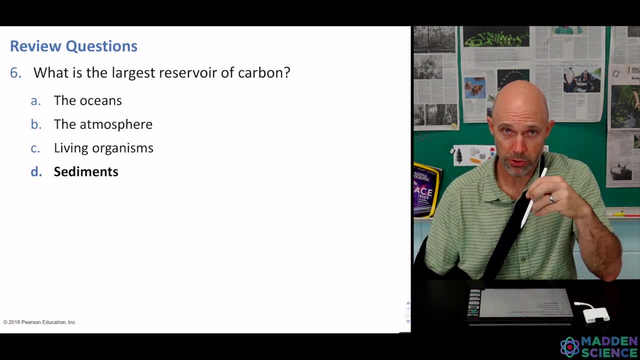 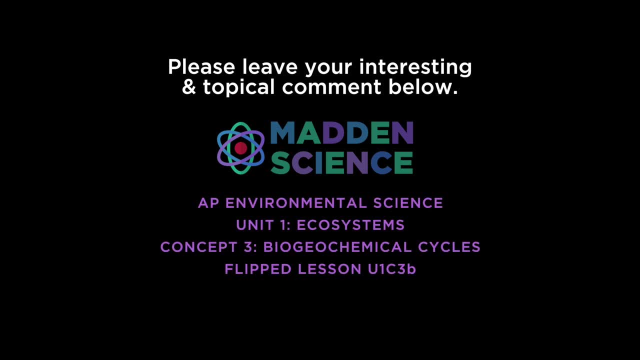 questions. Let me know if you have any questions and don't forget to post your interesting and thoughtful comment on the bottom. See you guys later you.